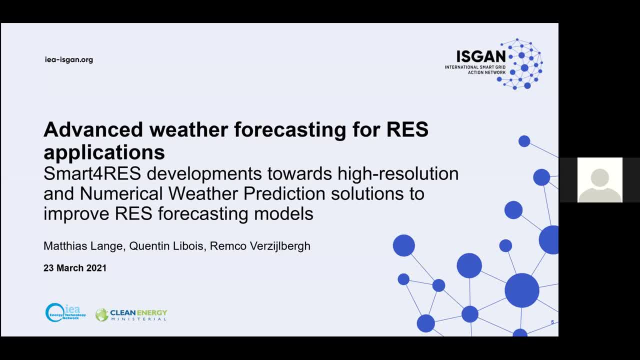 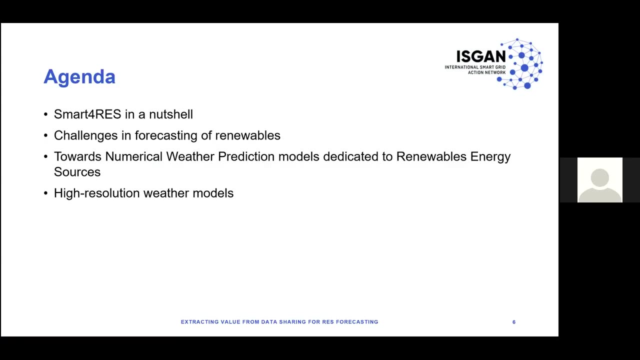 power predictions And, as I said before, Quentin and Remco will introduce themselves. My background is I'm a physicist. I did my PhD on wind power forecasting, but that's already several years ago. The agenda for today. I will very briefly tell you what Smart4S is. It's a new. 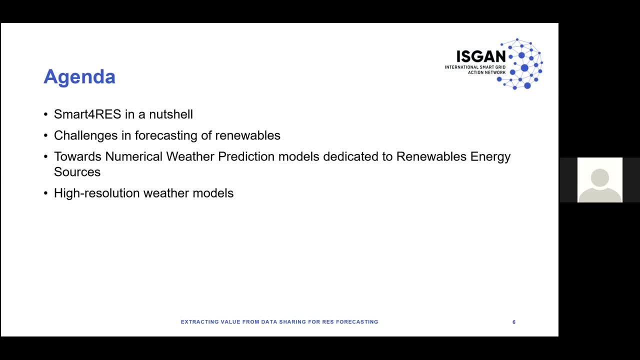 project and I will just briefly go into the details, what we're doing. Then I will highlight some of the challenges in forecasting of renewables that are closely related to today's topic, Which is a view on the more details on the numerical weather prediction models and high. 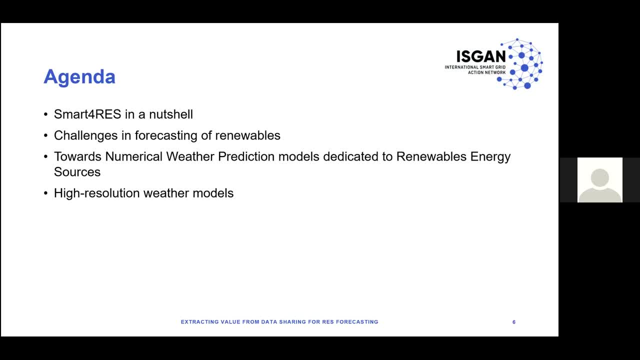 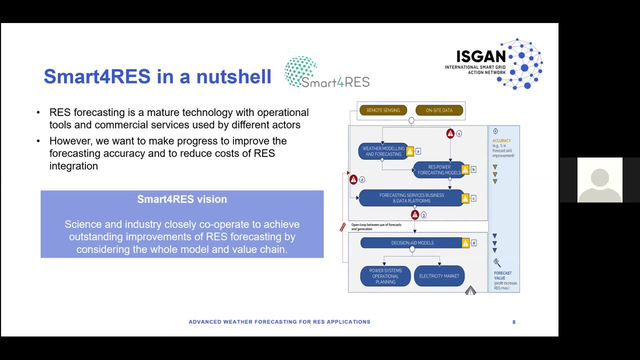 resolution weather models, But the real experts will be Quentin and Remco, and they will later on go into these details. So Smart4S is a Horizon 2020 research and development project, So it's funded by the EU Commission And the starting point is that we want to make sure 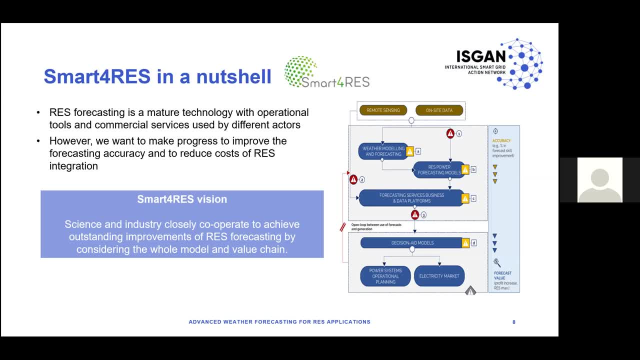 that this project is in high demand. We have a mature technology to produce wind and solar power forecasts. These services are established, So maybe also some of you use these forecasts in the daily business. So it's a completely mature product in the sense. 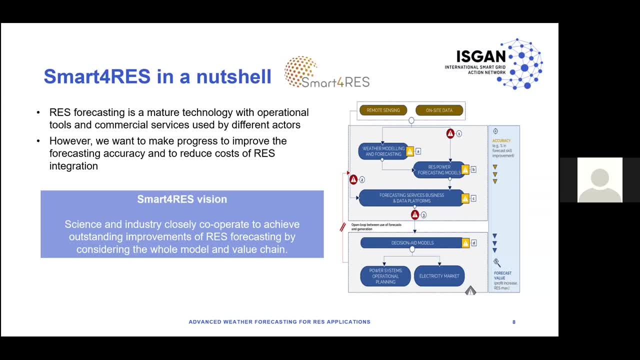 that it is already quite good. The forecasting quality is good enough to place bids on the market to do growth. I think the most important thing is to make sure that you are working with the right people, And I think that this is a really good opportunity for you to make sure that you are working with the right people. 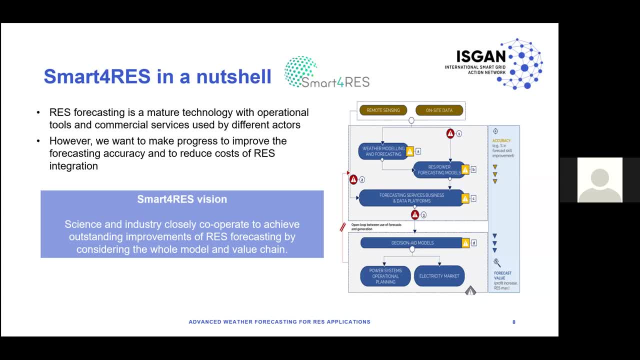 grid operation based on decision-making with forecasting, so that we've been doing this for 20 years now, but we still want to make progress. We want to improve the forecasting accuracy and to reduce the costs of integrating renewable energies into energy markets and energy grids. So the vision of this project is that science and industry closely cooperate. 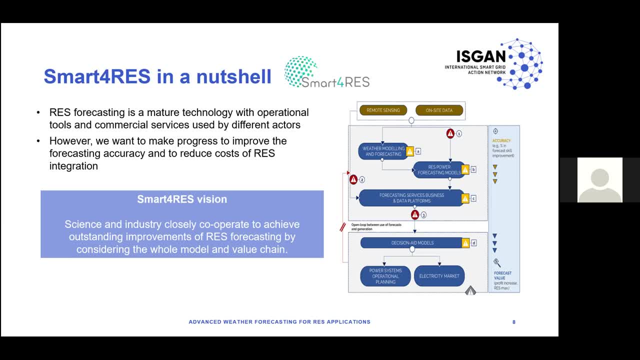 to achieve outstanding new improvements of renewable energy forecasting and that we look at the complete model and value chain And on the right-hand side you see this what we have in mind in terms of the value chain. So we have weather modeling and forecasting. 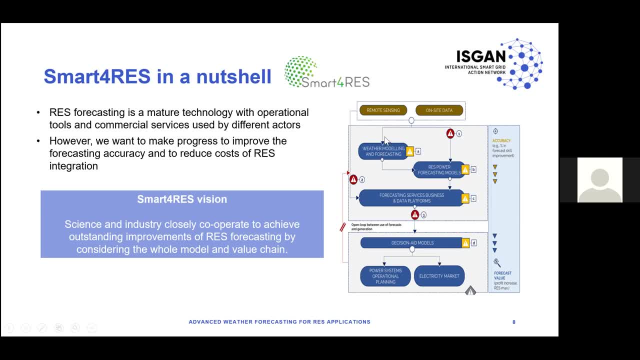 as one of the most important input data, and that's the topic for today. Then we have the power conversion. We have the business models and the data platforms that are necessary to really distribute the forecast and also to collect new kind of input data, And then we have special decision models for applications. 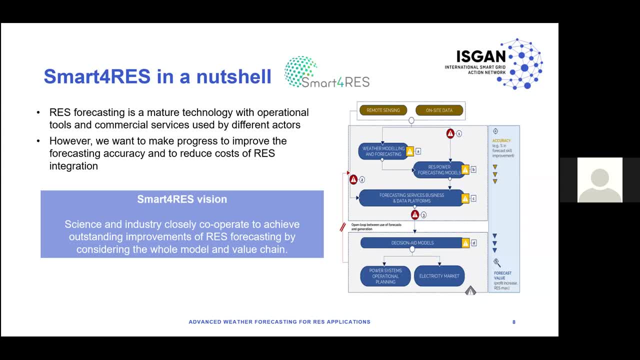 in power system operation and in electricity markets. So this is what we consider as the model chain, And the idea of these webinars is now to highlight aspects of this. So this is an overview of a smart fres webinar. We are live for one minute. 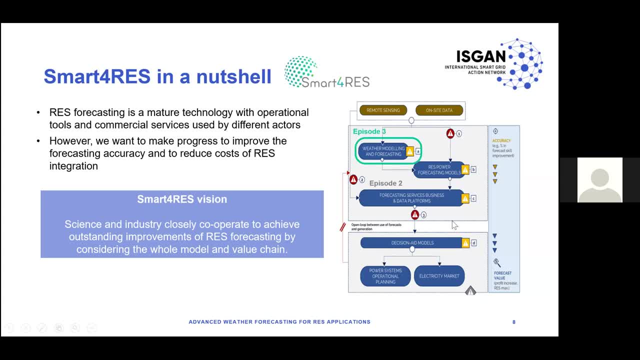 So the project has started one year ago, so we cannot provide many results at the moment, But we thought it's a good idea to share our knowledge at this stage already and to introduce what we have in mind. We are now in episode three, So these are two webinars on weather. 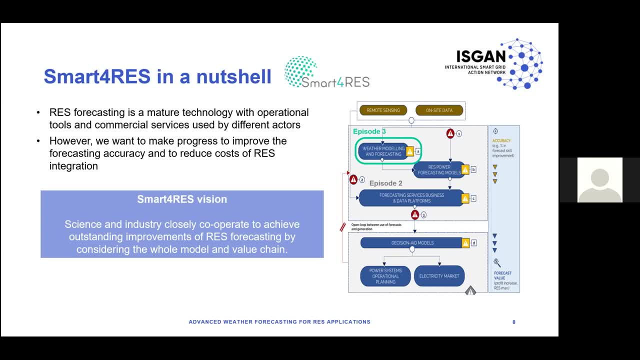 modeling and forecasting. This is part one and there will be. the next episode will be on the power conversion. So this is the plan. Here is an overview of the smart fres webinars. I'm telling you right now it's just an overview of the smart fres webinar, And then we will. 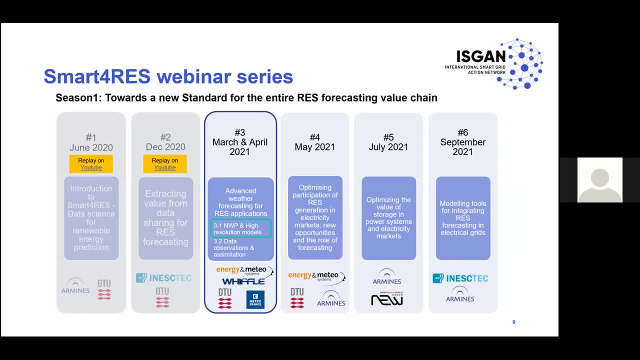 have a look at the kits to the next time, because you won't see us for that, And we will have a look at the next couple of minutes here. So this is the plan. Here is an overview of the Smart4S webinar series. As mentioned before, we already had two webinars In terms of Smart4S. 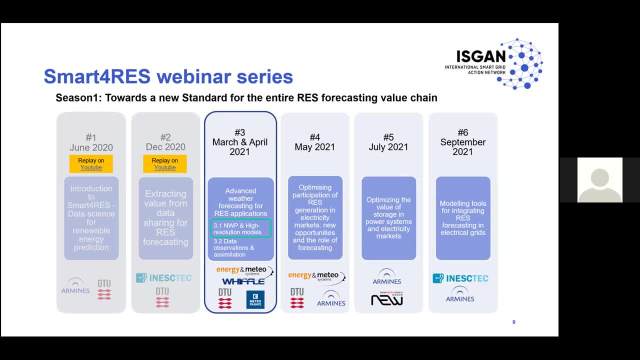 we're in episode three. You see the two parts- NWP and high-resolution models, today And at a later date. the data observations and assimilations will follow. Then we plan more seminars: episode four, five and six. So this is the plan, maybe more even if we come to a phase where we 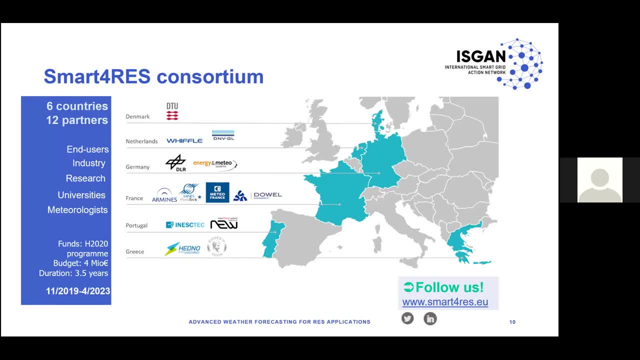 can show more results. The consortium is quite powerful because a lot of institutions and universities, also companies, are involved that have experience with renewable energy forecasting, from different countries. six different countries, 12 different partners from the EU: Quite a very strong consortium. 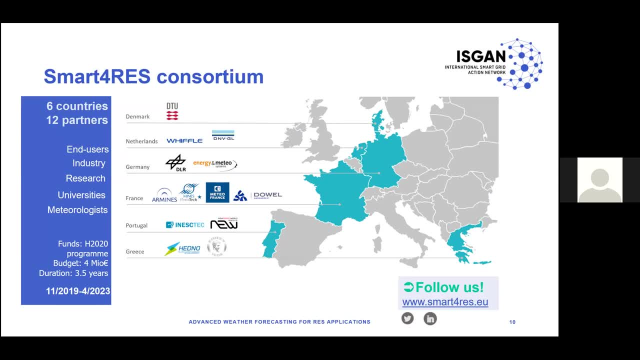 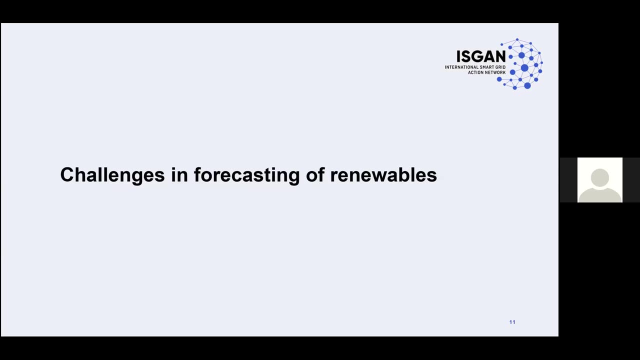 With a lot of experience. The project duration is three and a half years, So we have two and a half years to go to produce some good results, And what I wanted to say now is, yeah, some motivation. Why is it so important to look at the weather models? And I picked out 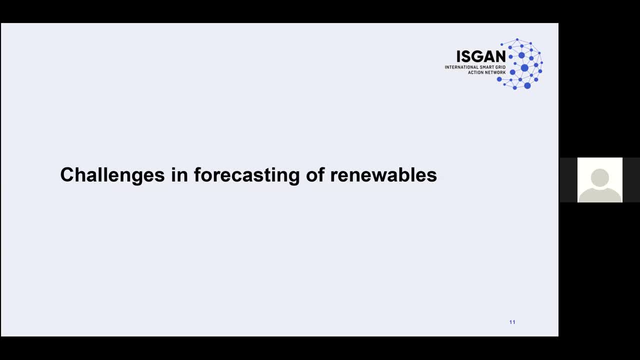 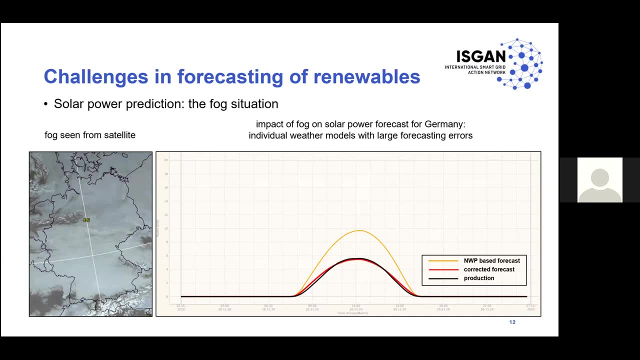 two examples, one from solar and one from wind power, to illustrate what today's challenges are. So let's start With solar power, And it's a very special situation related to fog. On the left-hand side you see a satellite picture of Germany with a high coverage of fog at this specific date. 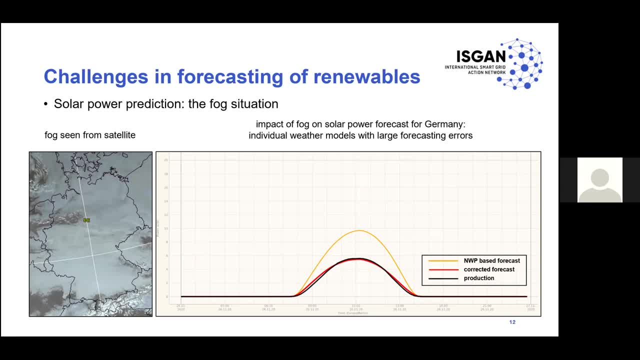 And this is nice to see on the satellite. but it's horrible to forecast this because the weather models. so the simulation of the atmosphere that tells us how the weather situation will develop in the next hours, In the next few days, has difficulties with fog to be, to have the precise amount of fog at the right. 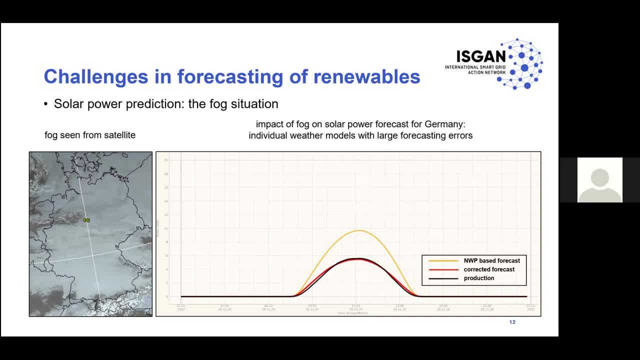 location at the right timing. So what you see on the right-hand side is a forecast for Germany, the aggregation of the German PV plants, And this is an intraday forecast. And you see, yeah, this is one day, obviously, And what you see in yellow or orange is the forecast for this day based. 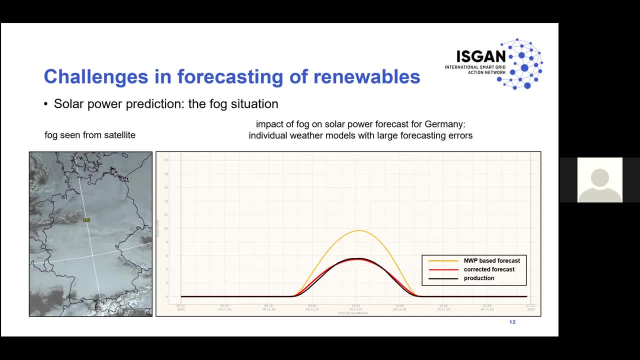 on the weather models only. So this is what not only one weather model but a combination of weather models thinks is the solar output of this day. And if you look at the black line, the production, you see that there's a big deviation. So the fog? 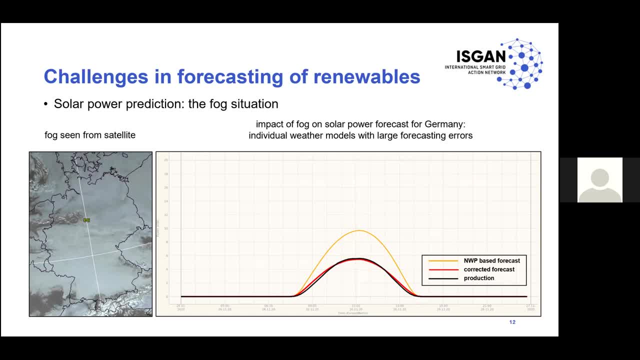 was thicker or heavier than expected And the power output was dramatically less than expected, than forecasted by the weather models. So what you see here is also the red line. that is the corrected forecast that we provided. So this is the forecast that we provided to our customers, but it involves some expert knowledge. 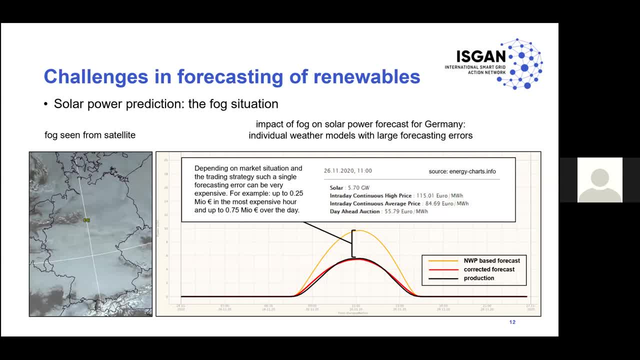 some extra knowledge on the weather situation. But if you look at this forecasting error based on the numerical models, then you could estimate this with RMSE, with MAE, the standard error measures. But what is mainly more important for the customer is to look at the euros he has lost And then how much. 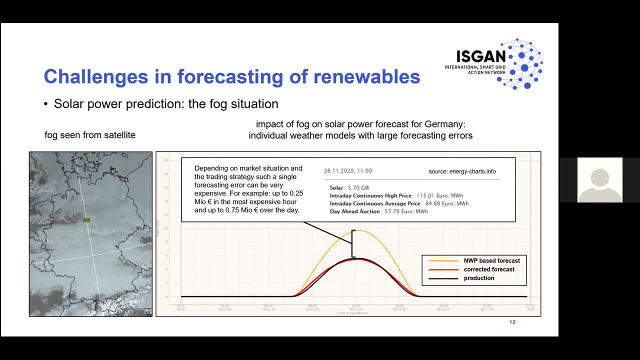 how expensive this is. how much money you lose depends on the trading strategy, of course, But you know, just as a rule of thumb, if you have a day ahead, if you had a day ahead, trade and then you have to. 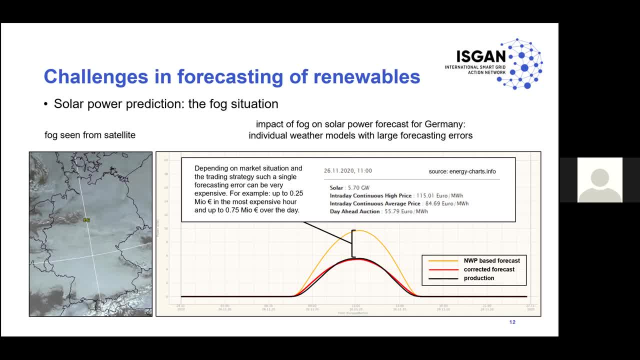 rebuy this energy from the trading perspective. you're short of energy. you have to buy this energy that is missing can be very expensive, ranging from a quarter of a million euros for the most expensive hours to about three quarters of a million, so 750,000 euros for the whole day. 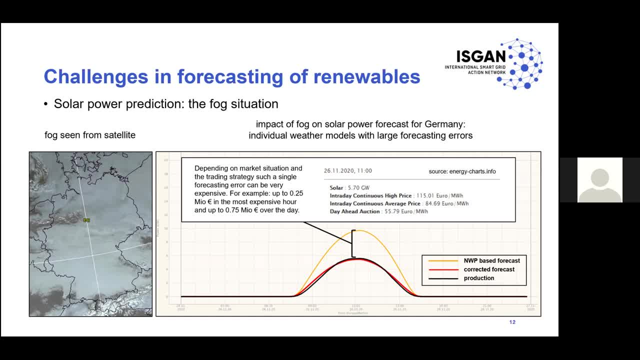 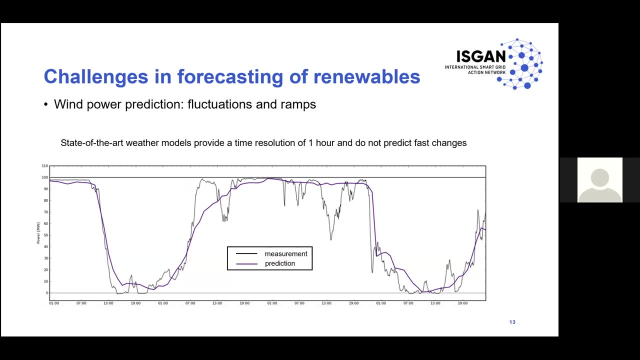 That's just an impression, It's. it can be expensive at single days if, for example, there is a forecasting error that occurs due to the weather model, for example. Second example is wind. What you see here is a wind power forecast for a. 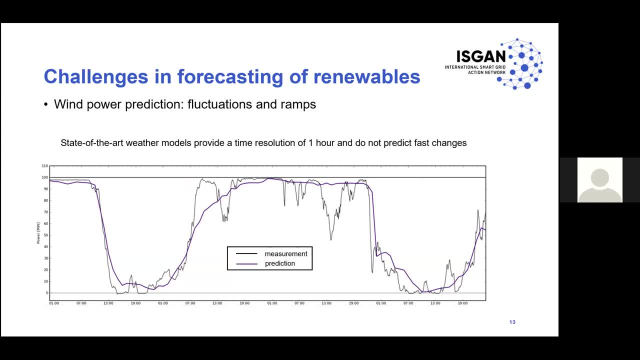 single wind farm. It is a good forecast. So what you see is the, the bluish line, the prediction and the measurement, and the measurement is obviously more fluctuating, But if you look at the general shape, it's a good forecast. over these hours that you see in this plot It's 100 megawatt wind farm. 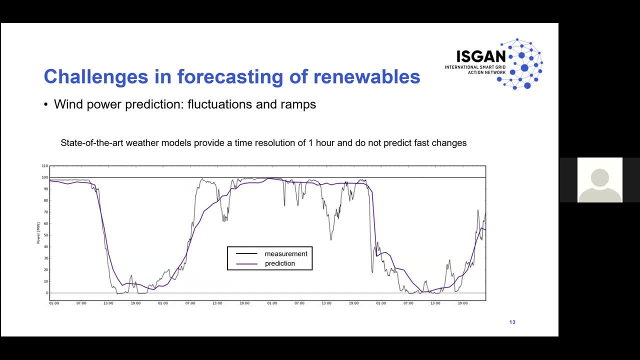 so the amount of errors is state of the art, I would say. But what you, what you also see, is that at certain positions, certain times, there are big fluctuations which are not covered by the weather model, not covered by the prediction. And these are the details that are coming. 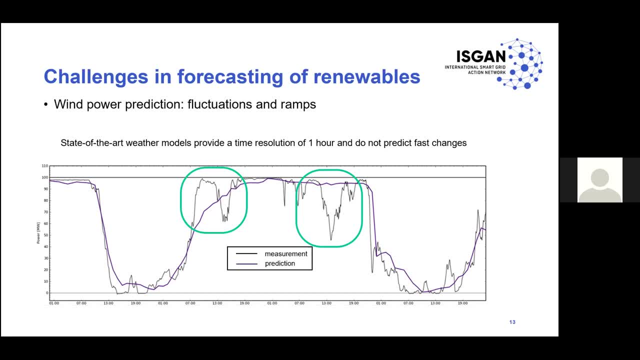 becoming more and more important. So this is essential to make progress on phenomena like so the fog for solar, the fluctuations for wind, to put more effort in the numerical weather models and then get a better power forecast for this. Okay, now I will hand over to Quentin. 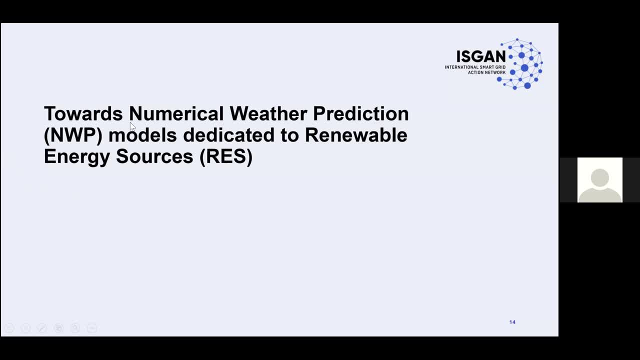 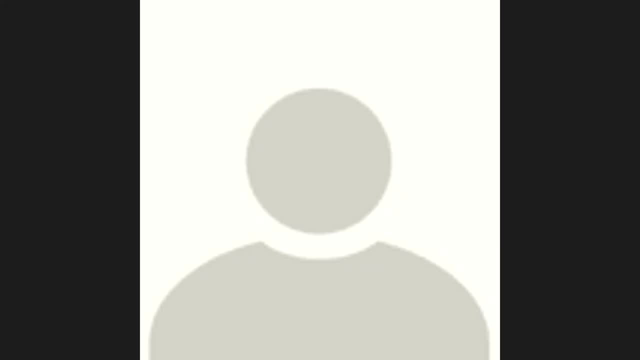 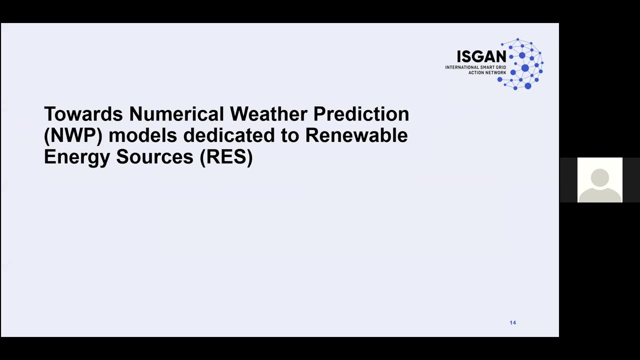 who is one of the real experts for the numerical models. Thank you so far, So thank you. Thank you, Mathias, for the transition. So my name is Quentin Iboa. I'm working at Meteor France, which is the French meteorological service, and they are mostly working on atmospheric. 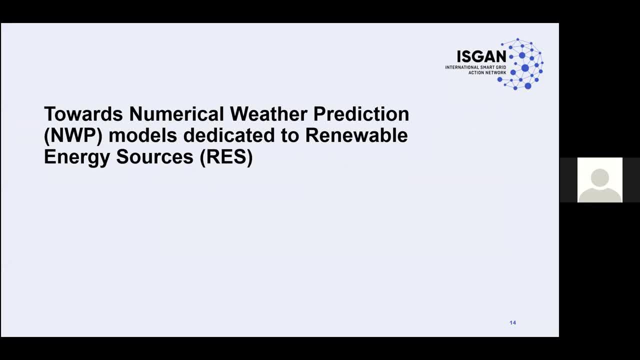 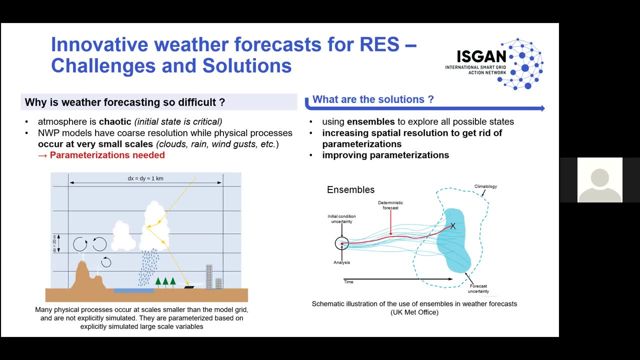 radiative transfer, And today I'll try to show how numerical weather prediction models- that I will now call NWP models- can help tackle the issues raised by Matas. So the first question is: why is weather forecasting so difficult? An easy answer is that the atmosphere is chaotic. 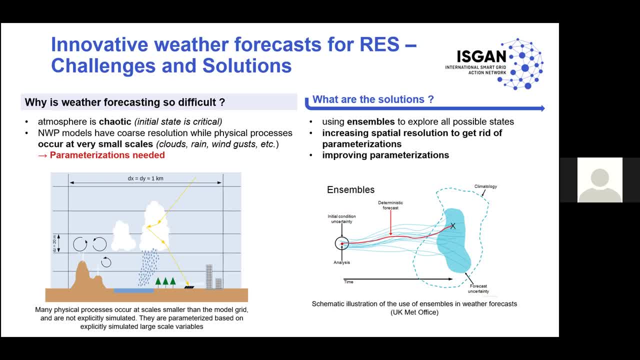 which means that the evolution of the atmosphere and its final state critically depend on the initial state of the atmosphere. In addition, NWP models have a quite coarse spatial resolution. It's roughly one kilometer in the horizontal and a few tens of meters in the vertical. But they try to represent 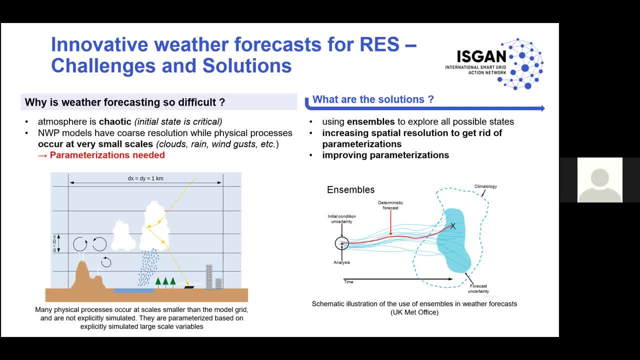 physical processes that occur at much smaller scales. For instance, if you think of clouds, of rain droplets, of wind gusts, of the interactions between solar radiation and clouds, or solar radiation and solar panels, if you think of the interactions between turbulence and wind turbines, it occurs at a scale of a few meters And, for this reason, 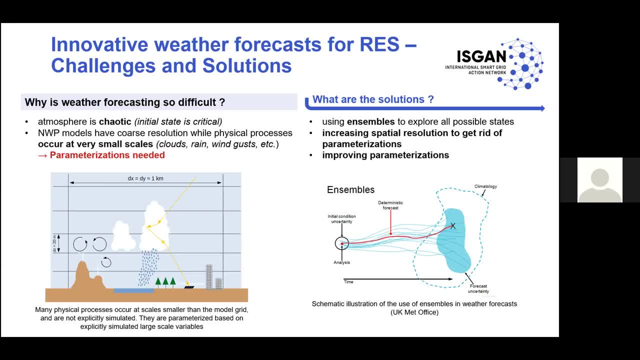 we need to develop and use what we call parametrizations which try to represent these subgrids, processes based on the large scale variables of the model. So what are the solutions Regarding these issues? to tackle the chaos issue, one idea is to use ensemble simulations. 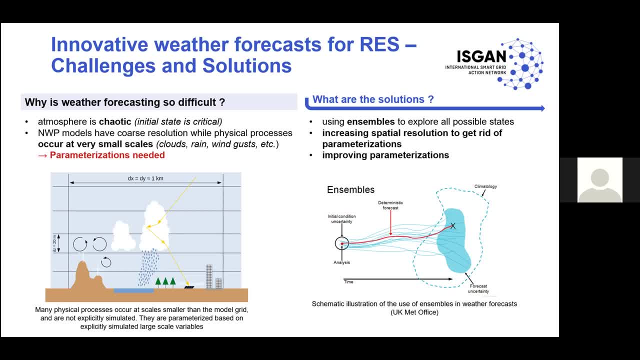 to explore all the possible states of the atmosphere. If you look at the figure at the bottom right, it's a schematic from the UK Met Office. You see that if you can start various simulations from slightly different initial conditions and look at what they provide, 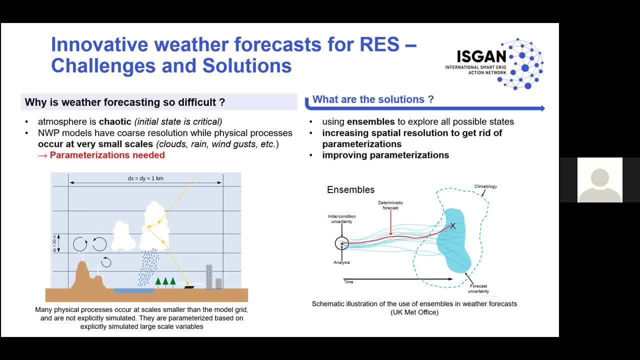 at the end of the forecast. the diversity or the dispersion of the forecast gives you a rough estimate of the forecast uncertainty, And this can be very useful, in particular compared to the case where I only used one deterministic forecast, which is symbolized by the red line on this plot, on this figure, which doesn't provide you. 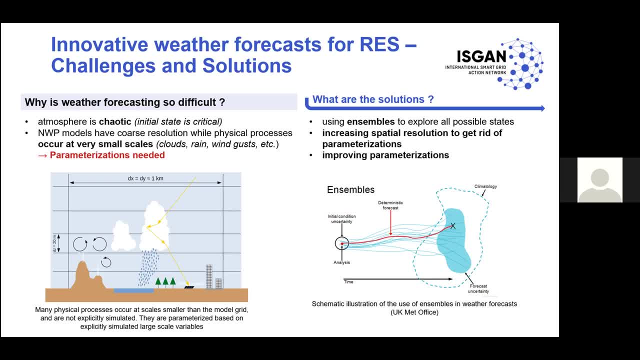 any information about the uncertainty. Another possibility is to increase the spatial resolution of the model to get rid of some of all the parametrizations that I just mentioned, And finally, it's also possible to directly work on the improvement of the physical parametrizations. So all these three strategies require quite a lot of work. So they are kind of 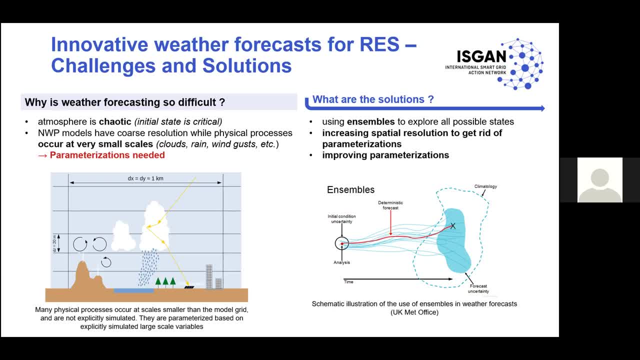 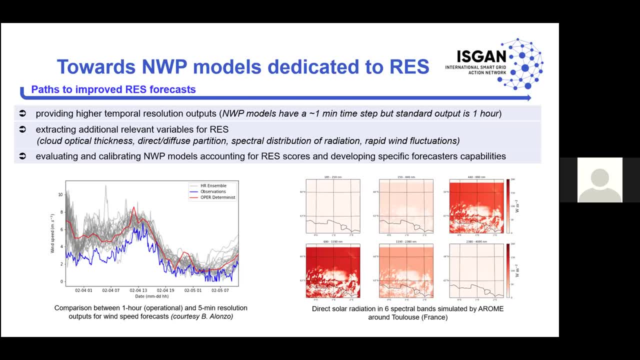 can be considered as long term strategies, But based on the current NWP models, it's already possible to think how they could be more dedicated to renewable energy production. First, as Matthias said, standard outputs of energy is one hour, But practically the internal time step of such a model is closer to one minute. 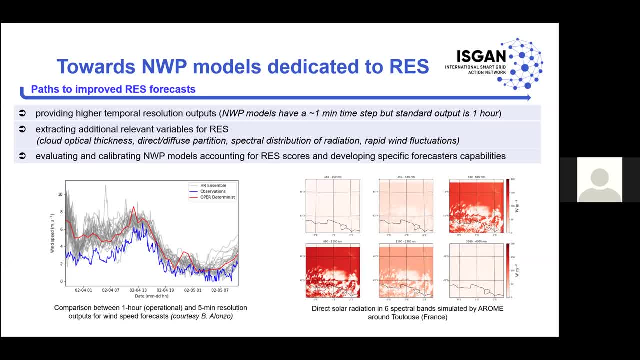 So it's technically possible to provide higher temporal resolution outputs from these models. The figure at the bottom left, which was provided by my colleague Bastien Alonso, shows the time series of wind speed measured at an atmospheric weather station. In blue you have the observations. 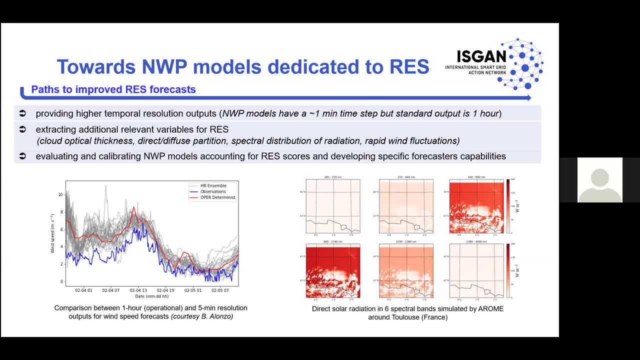 and in red the operational deterministic forecasts at one hour output resolution, And the gray lines indicate the various members of one ensemble simulations with outputs at five minute resolution And without getting into the details, what you can see is that the high frequency variations observed on the blue lines, which do not appear on the red line, they are captured. 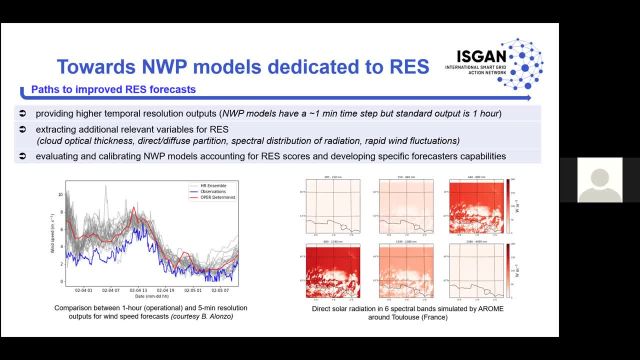 somehow by the gray. So it shows that there is some variability that exists within the NWP models that does not appear in the one hour standard outputs. Another venue is to extract additional relevant variables from the NWP models which could be relevant for renewables, For instance the rapid wind. 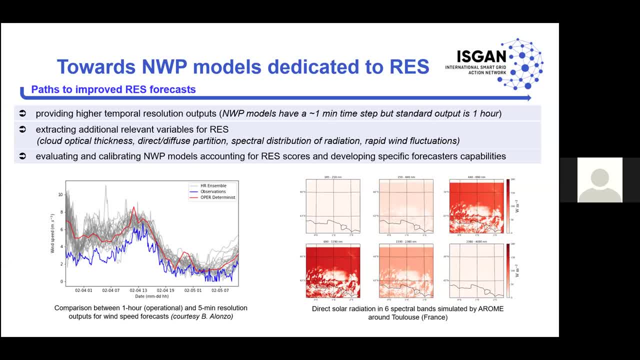 fluctuations or details about the cloud optical thickness, the details about the spectral distribution of solar radiation or the partition between direct and diffuse radiation, which actually exists in the model but sometimes are not outputs. The figure on the bottom right shows six panels. Each of the panels is a map around Toulouse in France, showing the solar irradiance. 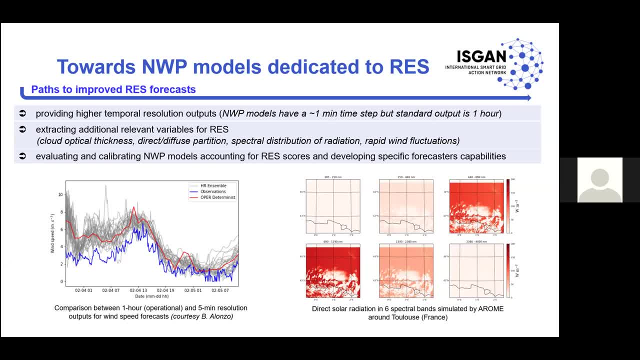 in six different spectral bands, And these six spectral bands correspond to the bands used in the relative transfer code embedded in the NWP model. And this kind of information can be very, very relevant for solar production, because the solar panels and their efficiency depend on the spectral distribution of the solar irradiance. 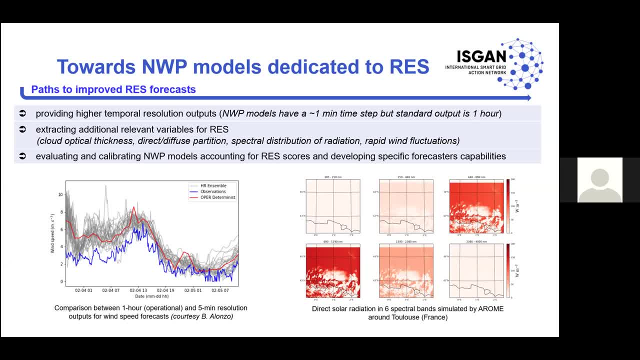 So extra information that you can get directly from the model without extra costs. And finally, it's worth having in mind that NWP models are evaluated against standard observations such as near-surface temperature and wind precipitation, and they are calibrated to best. 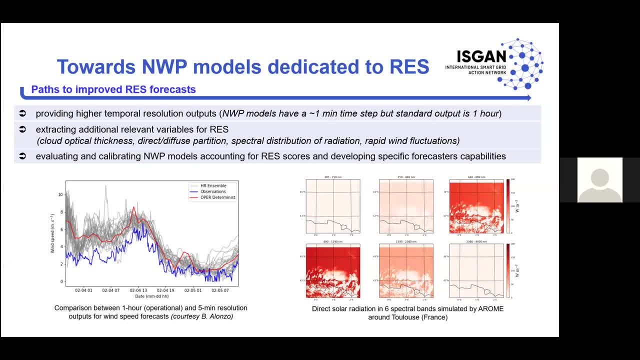 match these observations. We could think of models that would use, or would be evaluated against, RAS-relevant variables, such as wind at 100 meters high or solar irradiance, and which would be calibrated in order to best match these observations, And they would probably result in better models for. 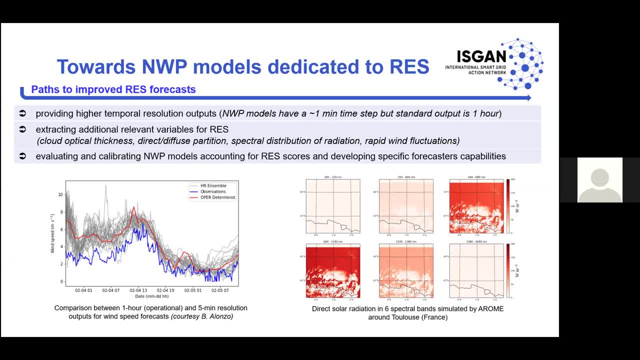 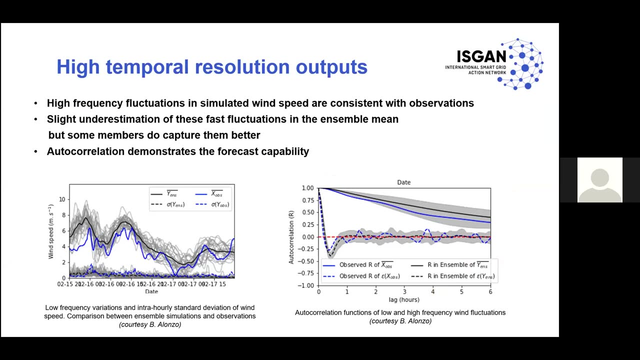 the specific use of renewable prediction. It's also worth considering training forecasters with specific capabilities dedicated to RAS. Let's now look deeper into the potential of high temporal resolution outputs. I show here again a time series of wind speed, comparing observations and ensemble simulations. 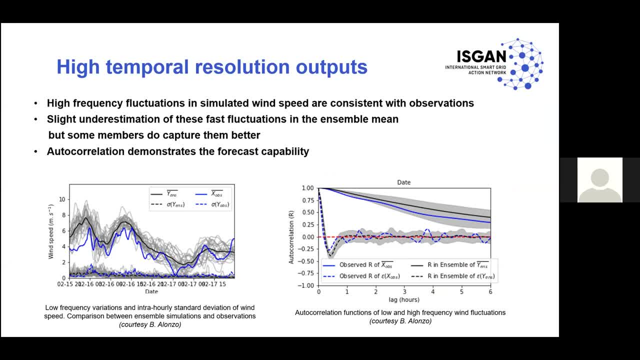 And in this case the wind speed was decomposed into slowly varying components, which is the upper line in the bottom left figure, and slowly varying well high frequency variations that are summarized by the standard deviation. intra-hourly standard deviation of wind speed at the bottom. 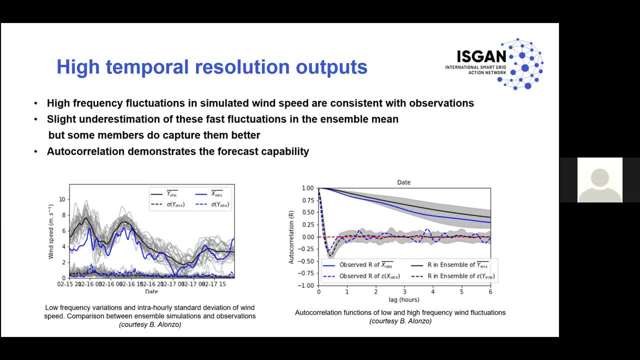 of the figure. In blue you have the observations and in black and gray the ensemble. On the bottom right figure I show the autocorrelation of both components, so the slowly varying wind component and the high frequency variations. This is again work by. 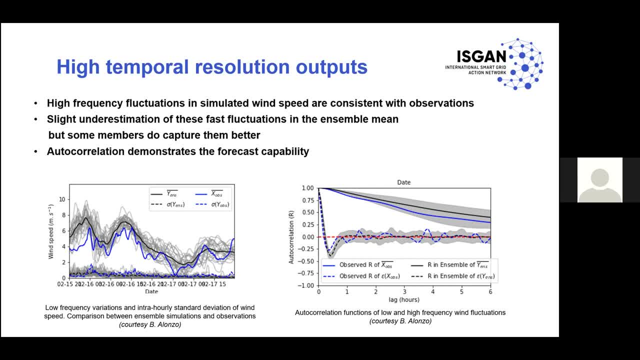 Bastien and Onzo. What this shows is that the high-frequency variations of the wind speed are the high-frequency fluctuations extracted at the five-minute output resolution are consistent with the observations. It's not only the idea to have higher resolution outputs, but to check that they. 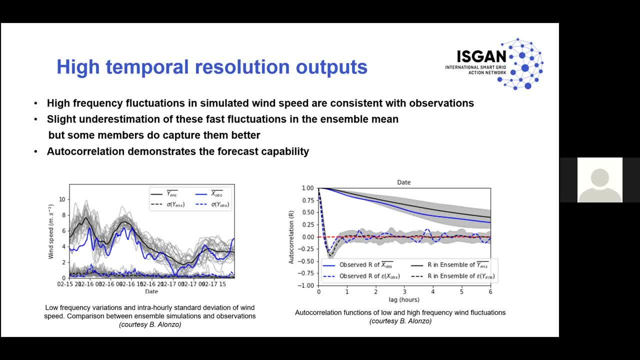 are physically consistent. There is an overall slight underestimation of the fast fluctuations in the mean of the ensemble simulations. It's the dashed black line in the bottom left figure. but some of the numbers do capture the high-frequency fluctuations. but it's not a given. 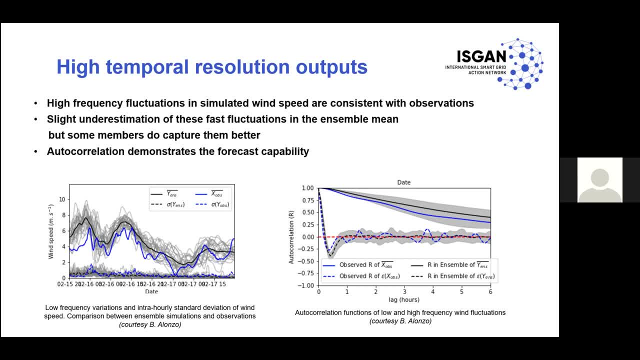 And finally, the match between observed and simulated autocorrelation shows that both the slow components and the high frequency variations are consistent between observations and simulations. So it seems, based on these illustrations, that the five-minute output resolution does contain some valuable information about high frequency variations of wind. 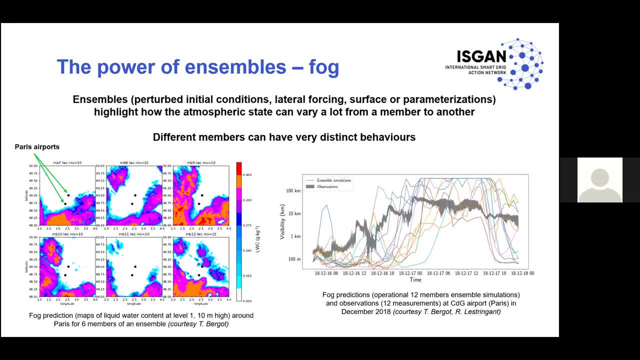 Let's now look at the power of ensembles, with a focus on fog. This slide is based on a work by my colleagues Thierry Pergaud and Renaud Lestringan. As I said previously, ensembles can be built from different initial conditions or by perturbing the lateral forcings in the case of a limited-area model. 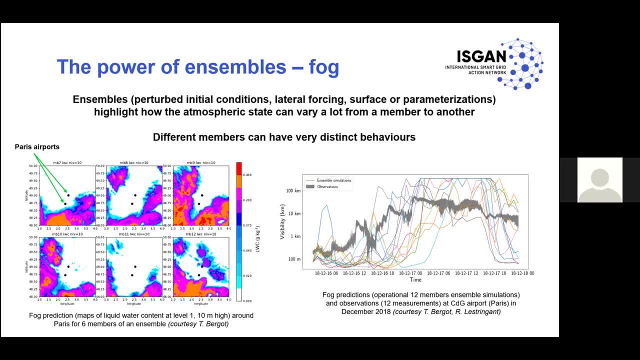 or perturbing the physical parametrization of the interactions with the surface And generally ensembles highlight how the atmospheric state can vary a lot from one member to another audience of the ensemble. The figure on the left shows six maps corresponding to six forecasts from six different members of one ensemble simulation around Paris. 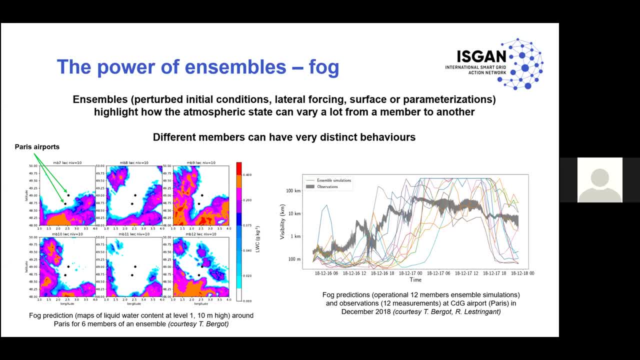 and the two dots in the middle. The color indicates the location of the Paris airport. The color indicates the liquid water content or, more or less, the cover of fog in the first level of the model, which is closest to the surface. I show this picture essentially to illustrate that among six different members the patterns and the intensity of the fog is very different. 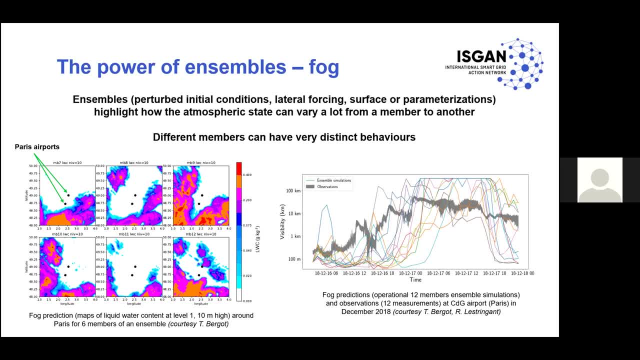 It shows that basically, in this particular case, there is a very high uncertainty on the occurrence and position of fog, And the curves on the right show the evolution along one day or two days of the visibility at Paris airport, Charles de Gaulle airport. 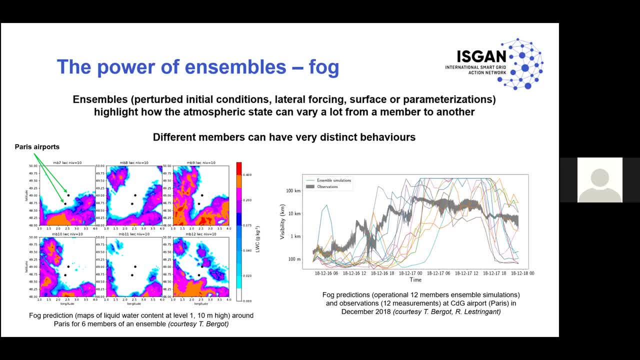 In gray you have the observations and the different lines correspond to 12 different members corresponding to the operational ensemble simulations performed with an AROM model at Paris airport. The idea is that when you have a drop in visibility it corresponds to the occurrence of the formation of fog. 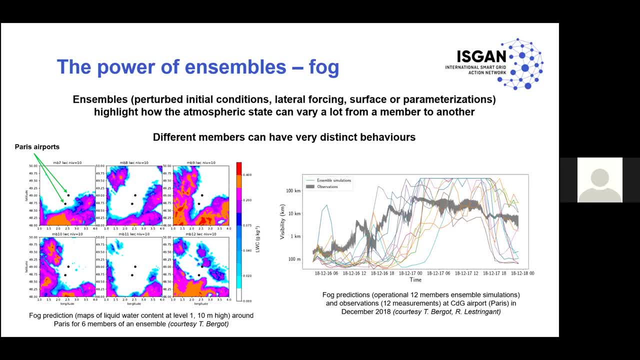 And what you can see is following different members. you see that some of them perfectly get the fog formation, while some others completely miss those. If you look at the first, at the beginning of the simulations, you have one single blue line which is completely missing: the fog events. 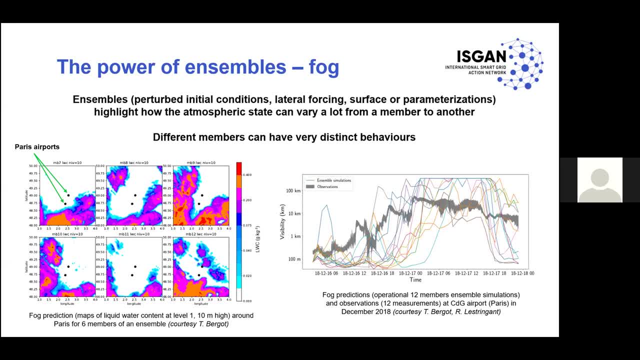 Sometimes the time of formation or dissipation of the fog is well captured, or not at all, by the different members. So it's essentially to illustrate that different members of one single ensemble, which are meant to represent the diversity of the potential states of the atmosphere, can have very distinct behaviors. 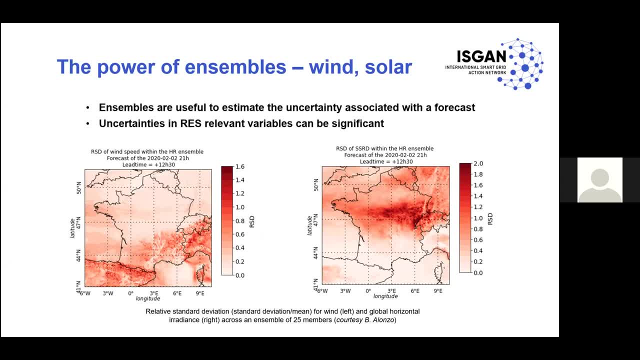 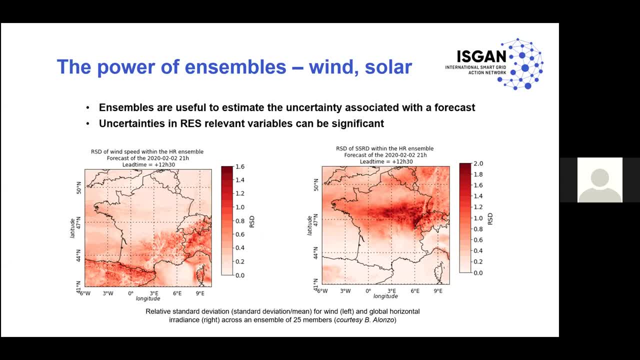 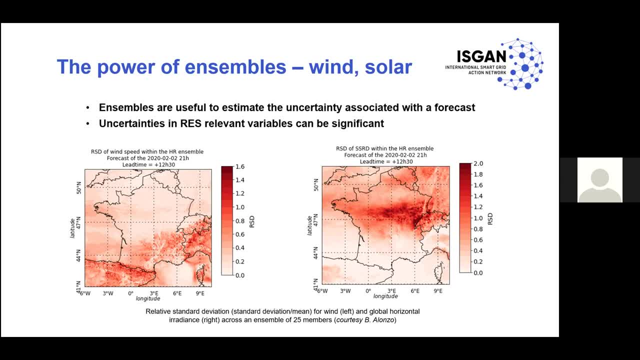 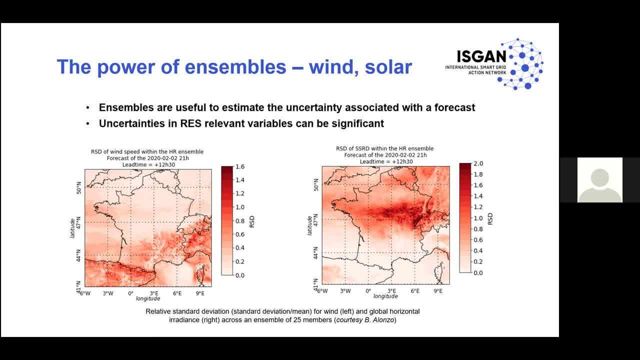 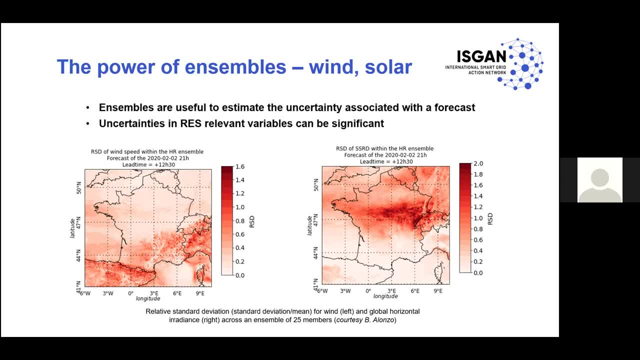 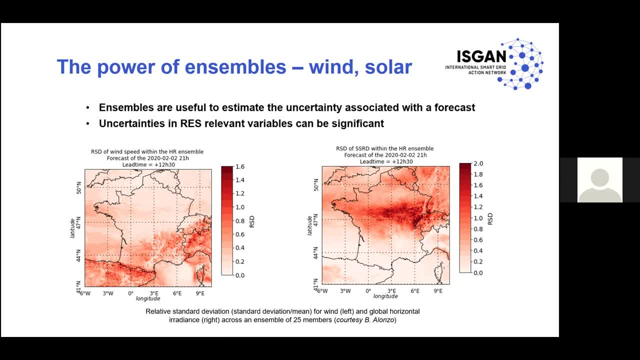 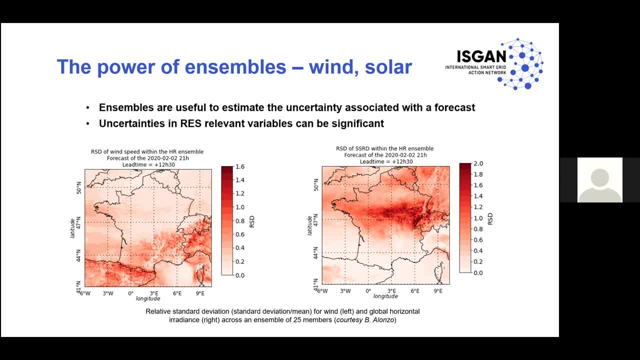 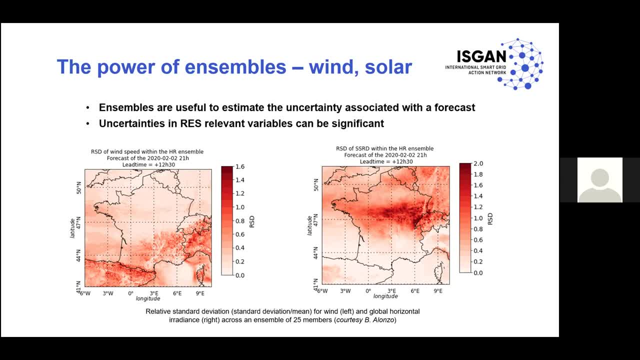 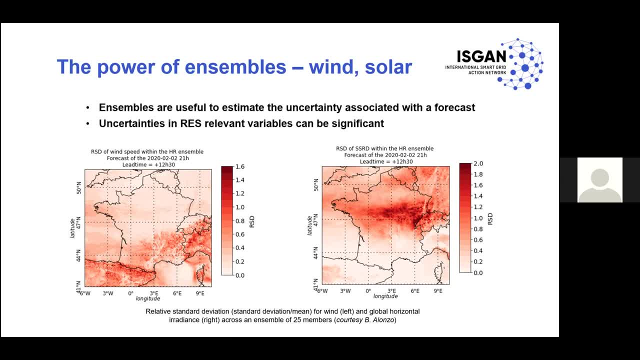 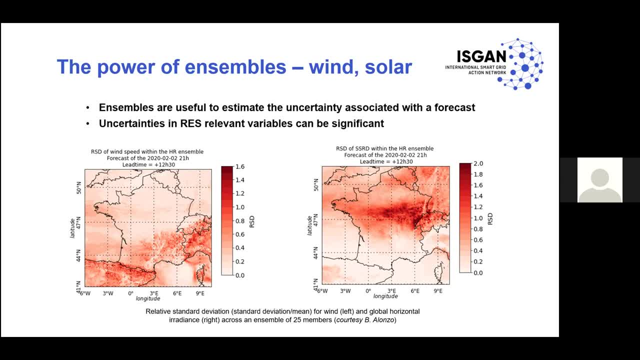 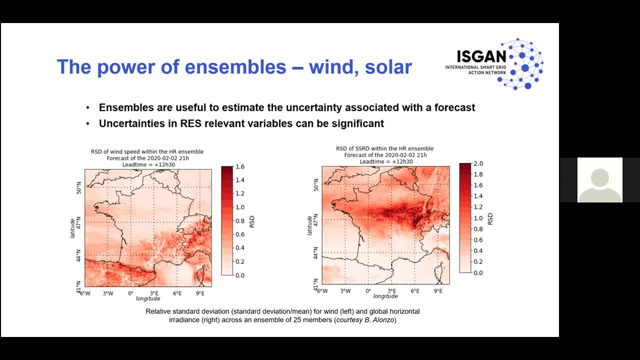 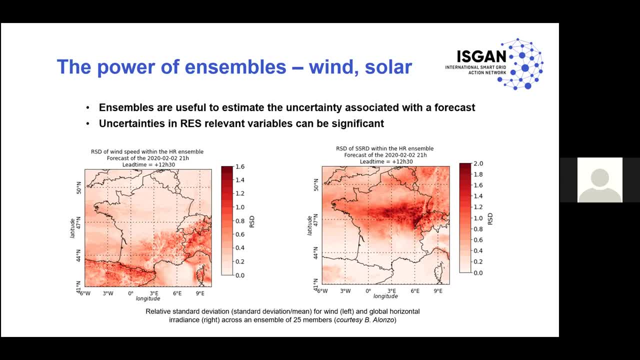 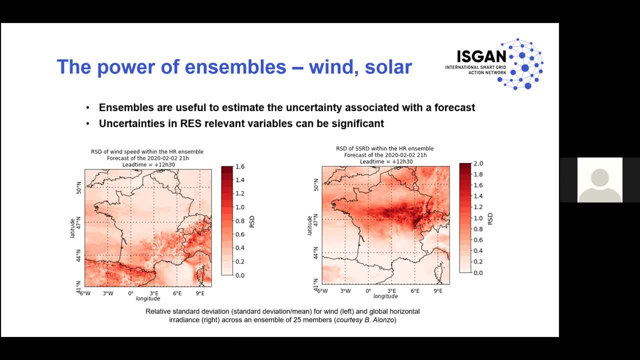 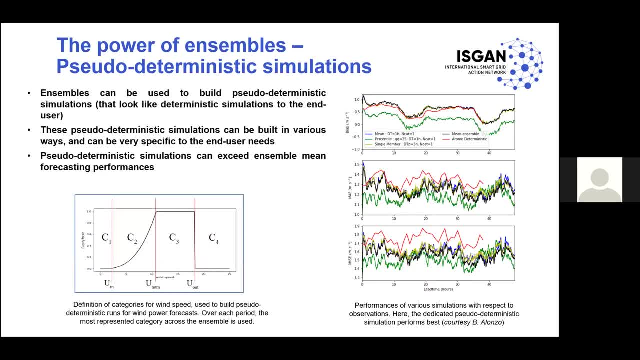 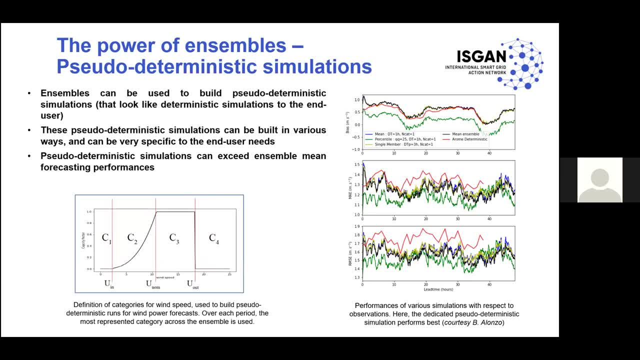 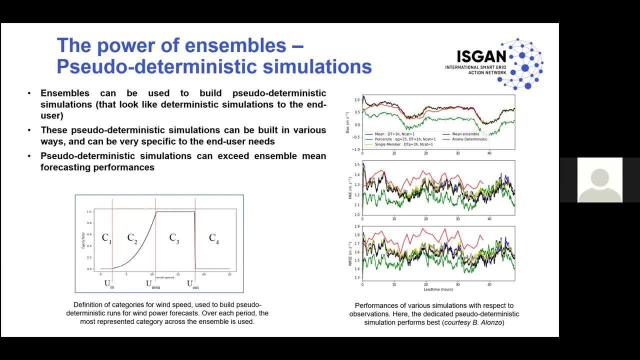 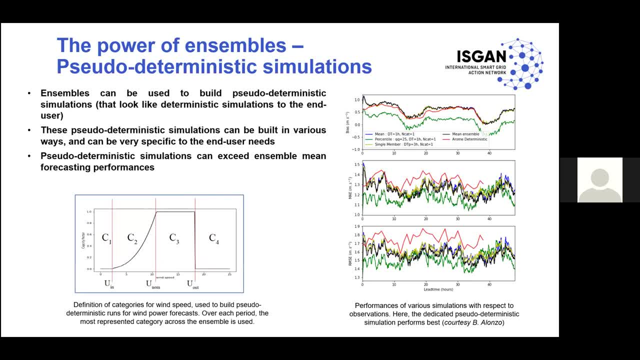 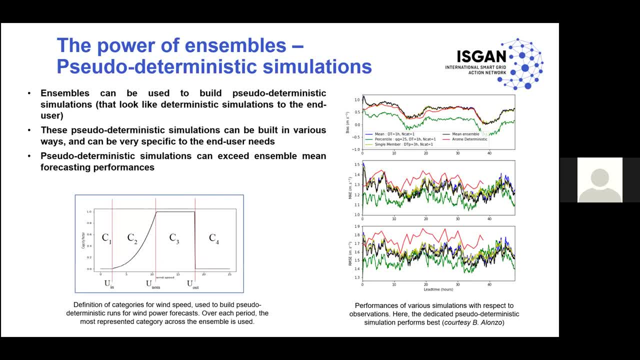 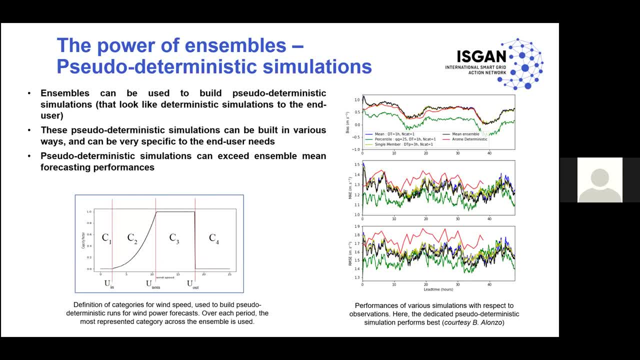 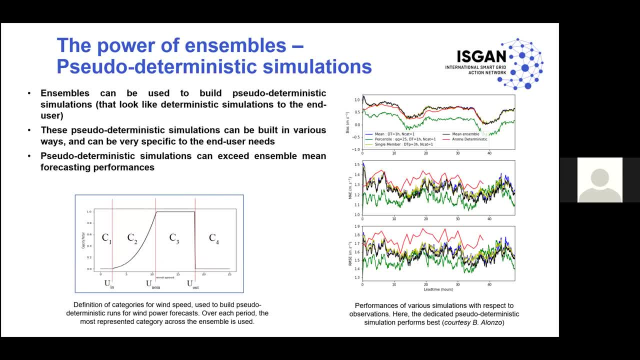 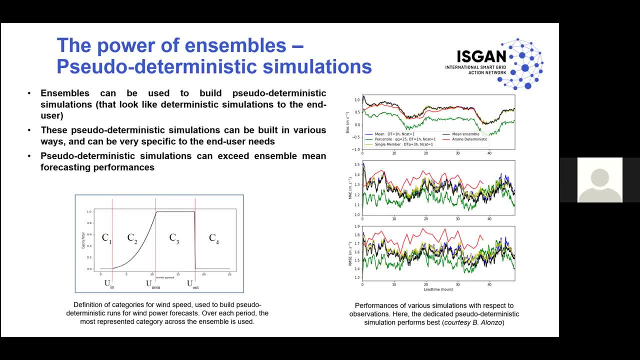 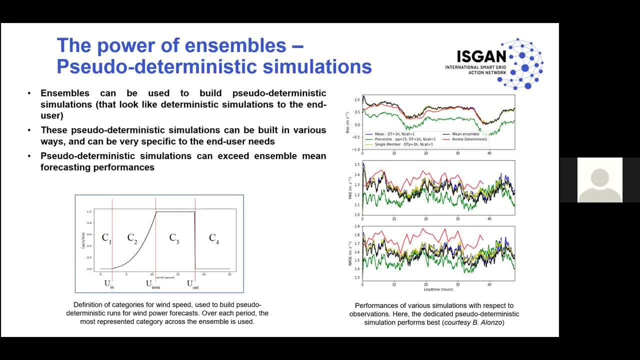 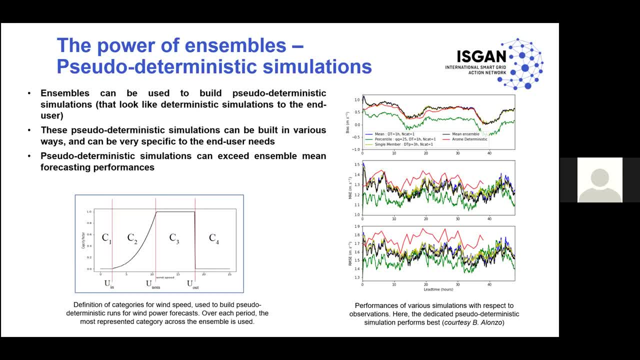 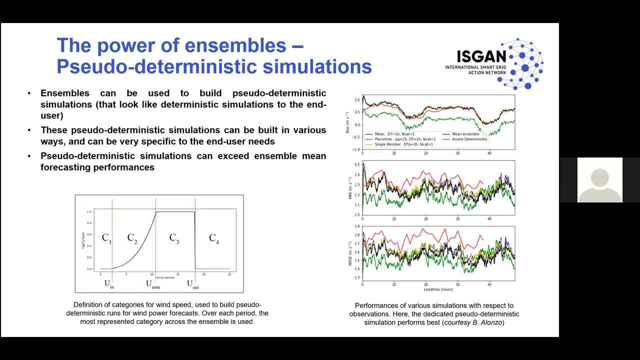 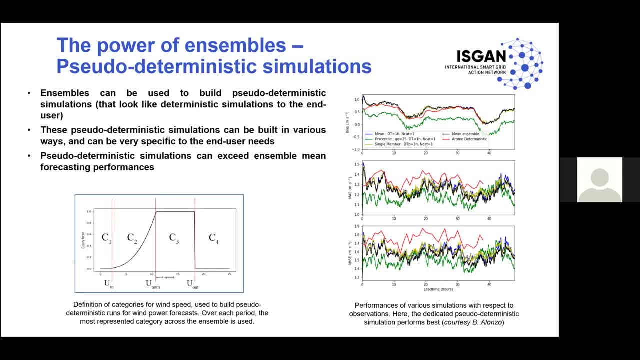 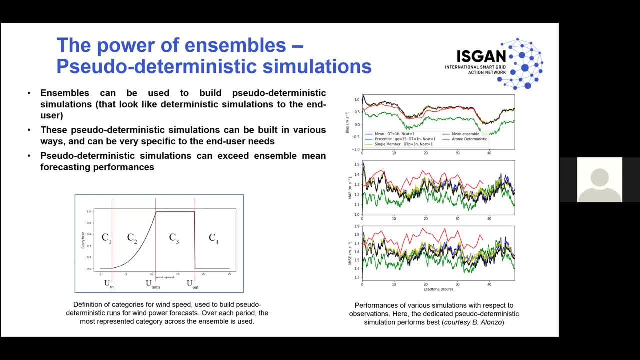 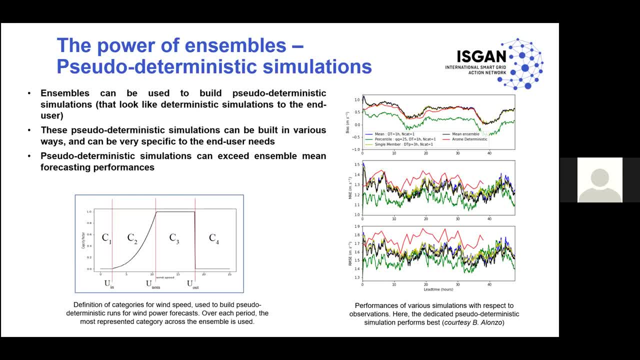 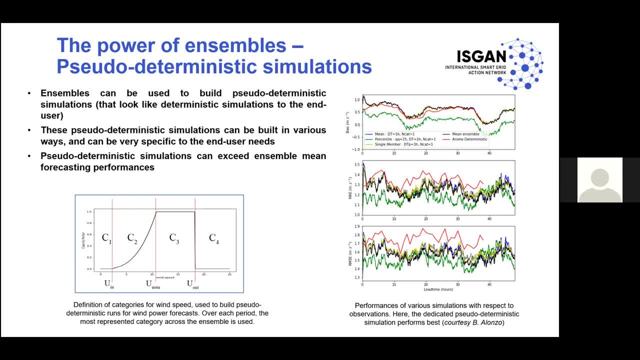 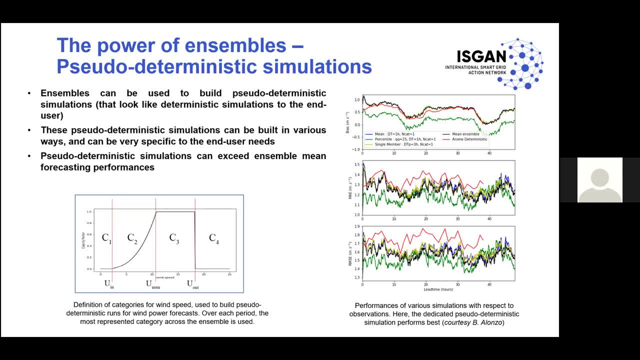 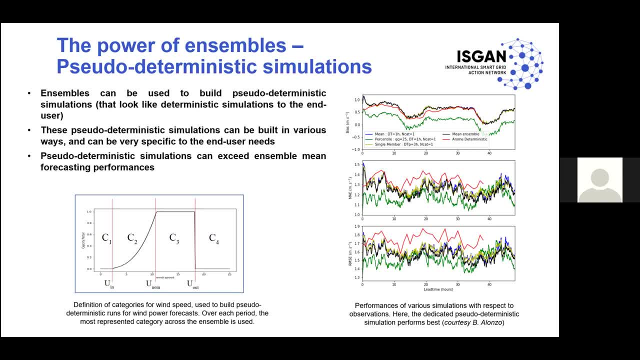 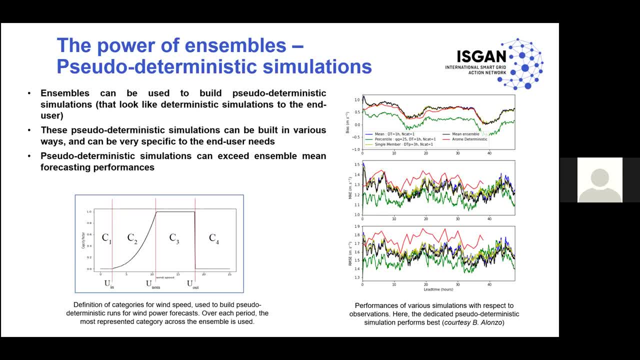 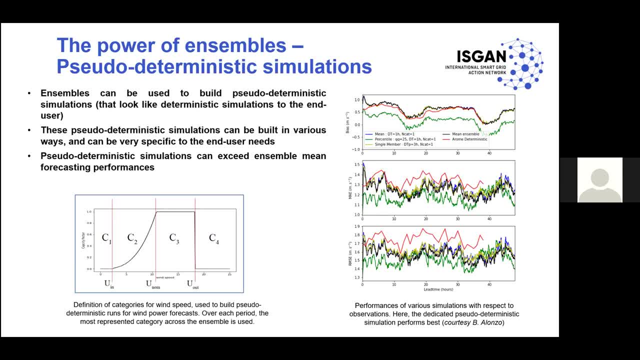 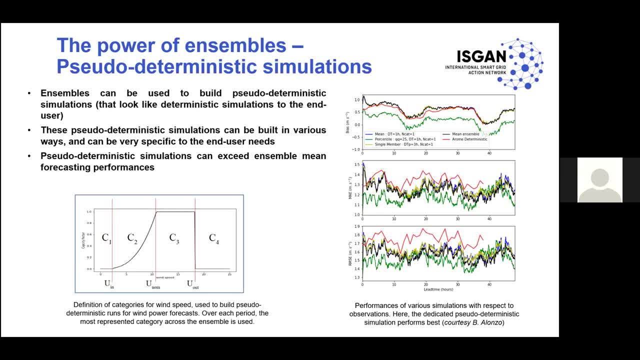 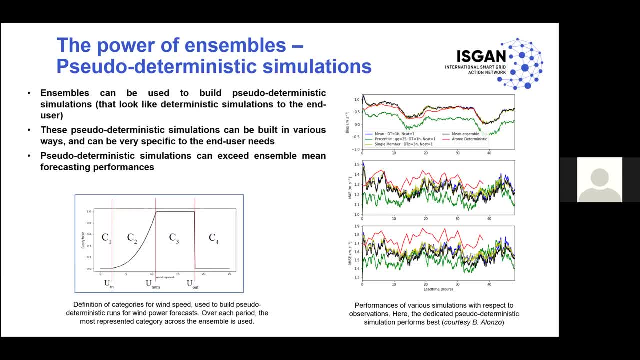 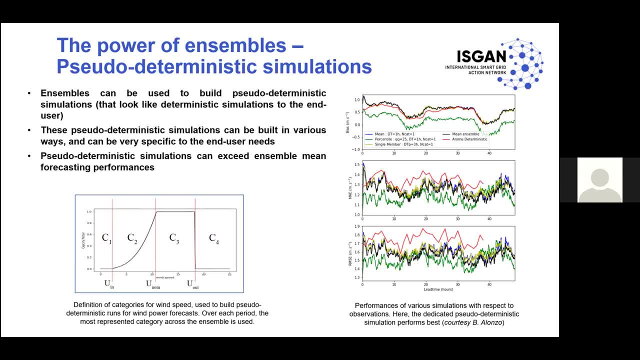 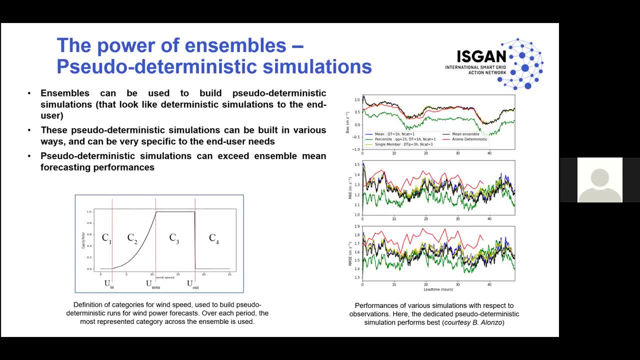 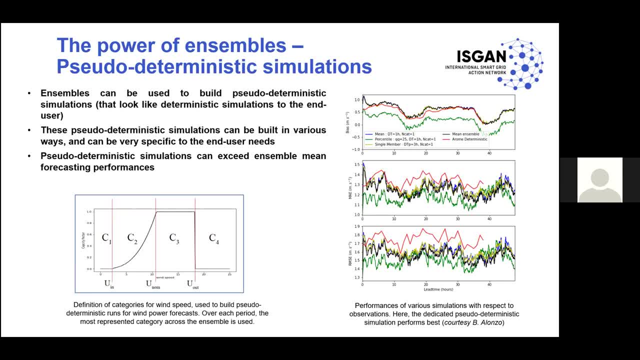 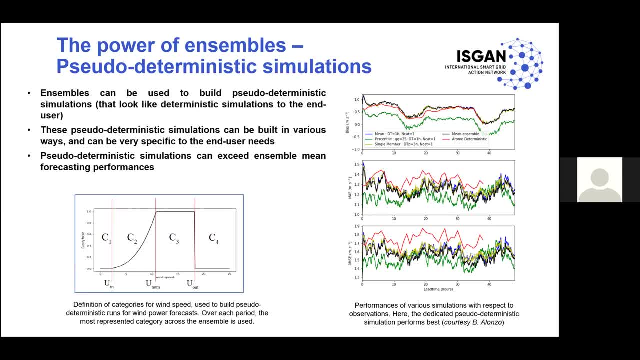 So, for instance, here I show two maps showing the relative standard deviation. We're now on the white table. At this time we're preserve all. the Hong Kong map version doesn't look in here, But it finally Iрав existed also. We haveósimulation. So in red you have the deterministic simulation, in black the mean of the ensemble And, for instance, in green the 25% of the most represented category And the 25% of the most represented category, which means that at each time step we select the member that corresponds to the 25% file of the category. 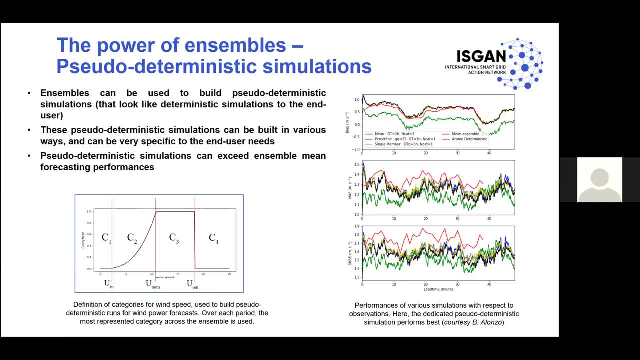 But choosing this pseudo-deterministic methodology with percentile 25 provides better results than ensemble mean and then deterministic simulation for all these three error variables. So it's just an illustration to show how, based on ensemble simulation, we can build pseudo-deterministic simulations. 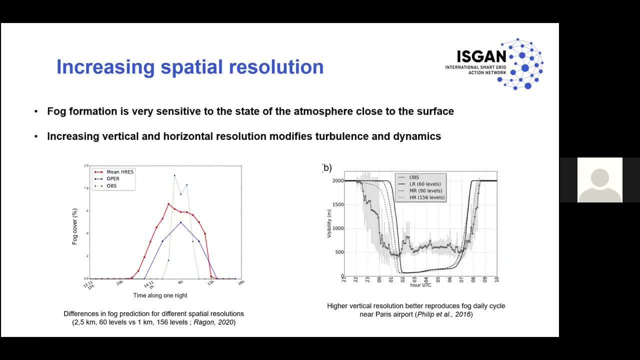 And finally, I'd like to show some results highlighting the impact of the spatial resolution on the forecasting of cloud of fog. On the left, you show one time series of fog cover observed in green and simulated in blue with the operational model and in red with the high resolution model. higher resolution. 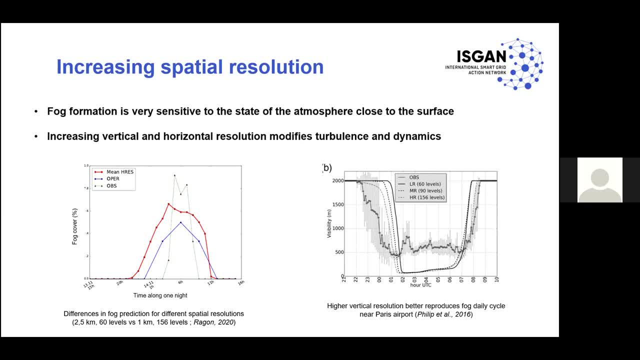 model And it shows that the two curves are quite different. And the difference between those two models is only the spatial resolution. It's getting from 2.5 kilometers to 1 kilometer in the horizontal and from 60 levels to 156. 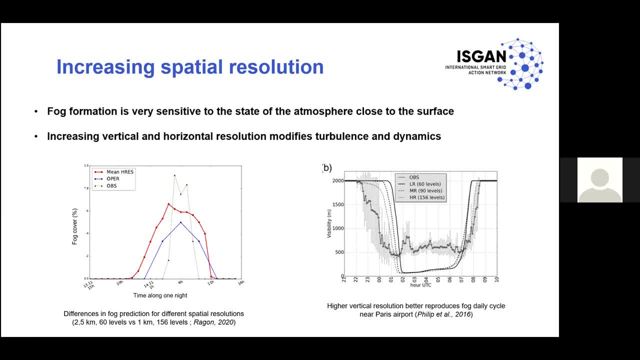 levels in the vertical. So it's essentially to illustrate that changing the vertical resolution in particular makes a big difference in how the model behaves And the prediction of fog, And this is again illustrated in the figure on the right, where the visibility observed. 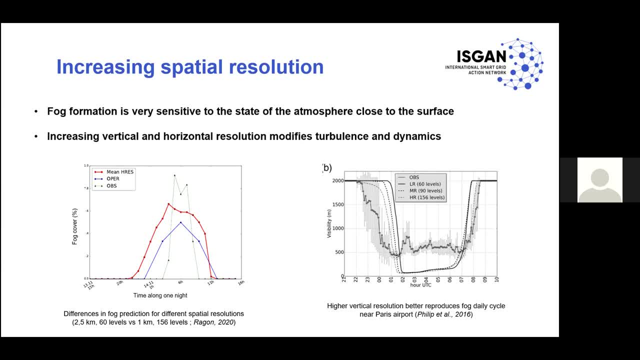 at Charles de Gaulle airport is compared to the visibility predicted at the north of the city of Sao Paulo. That's very interesting. Thanks by the model and you see that the high resolution simulations better captures the daily cycle of the fog, in particular the formation of cloud in the late evening and its dissipation in the morning. 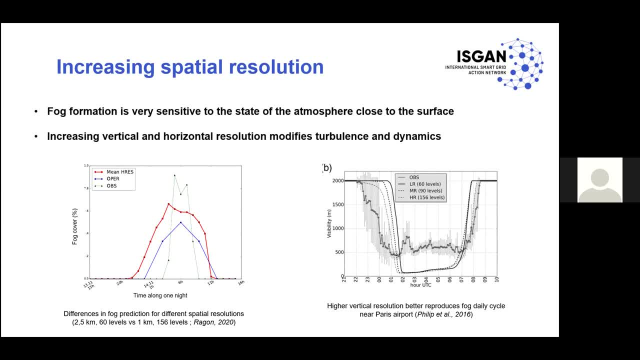 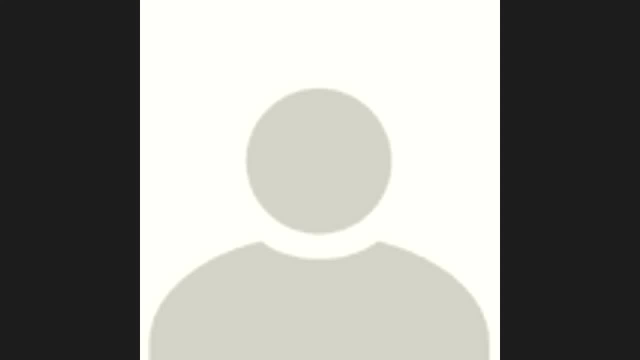 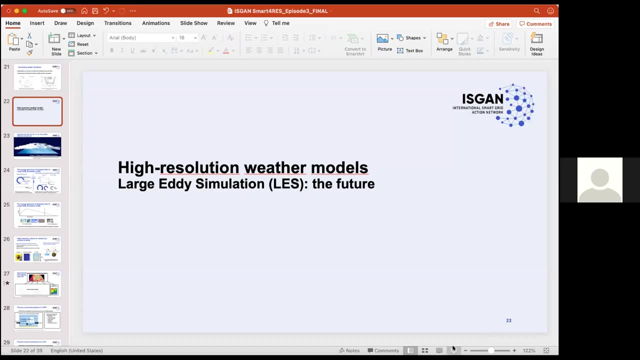 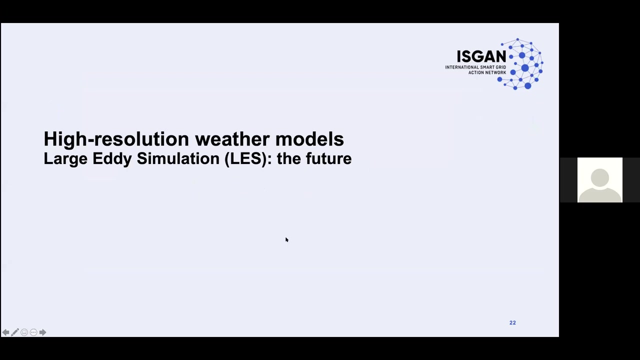 And with this I leave the floor to my colleague, Remco. All right, thank you, Quentin. Let me share my screen There. we go share and go to full screen. So, thank you, Quentin. My name is Remco Verzelberg. I'm with Wiffl, a weather forecasting company that 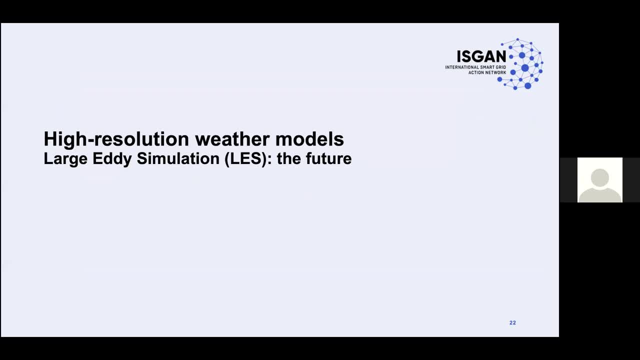 specializes in very high resolution weather prediction. I also have a background in physics and also energy economics At TU Delft. Wiffl is also a TU Delft spin-off. So I will talk a bit about high resolution weather forecasting with a particular technique called large eddy simulation, And I will just 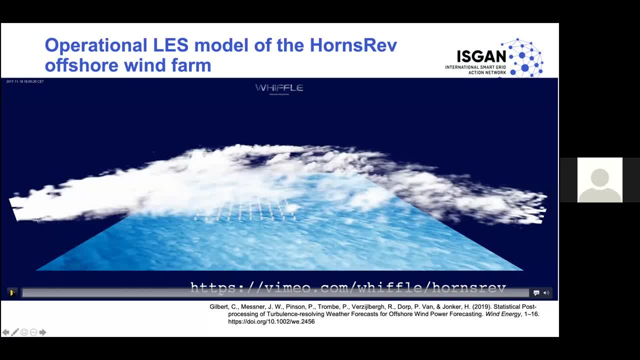 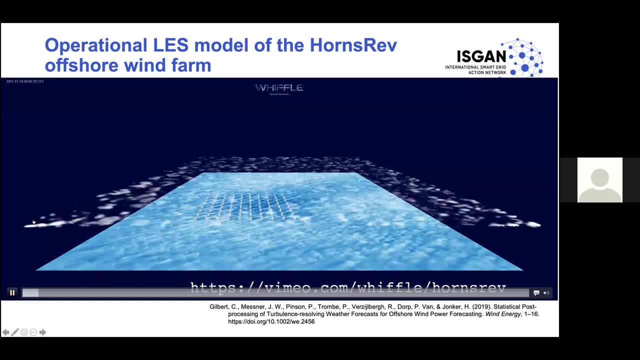 play this video so that you get a bit of a taste what it is, and then I will explain what we are seeing. So we are looking at a large eddy simulation based weather forecast for an offshore wind farm in Denmark, the Horntreff wind farm. 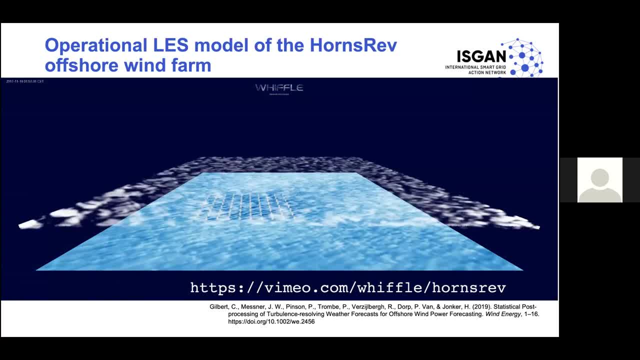 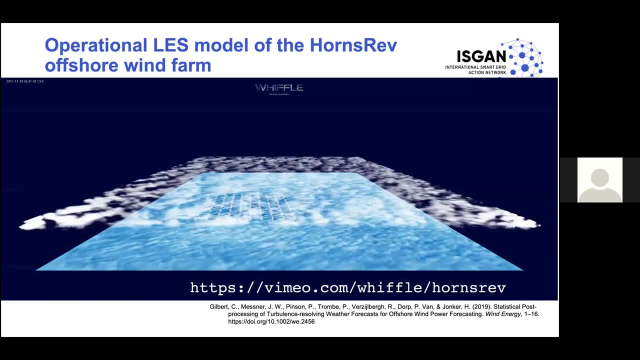 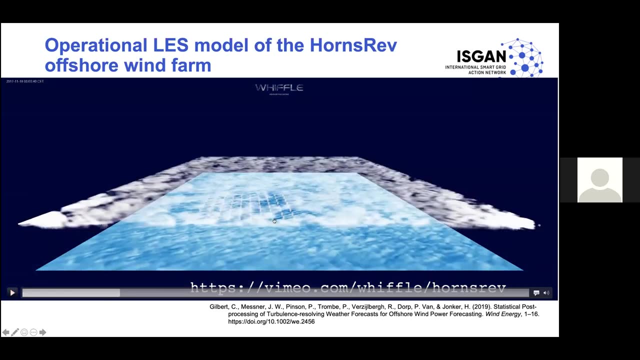 So you see this regular array of gray dots. Those represent the wind turbines. Now the blue colors represent the wind speed at the surface. So you can also see- I'm just going to pause it here for a moment- you can also see that behind the wind turbines there's lower wind speed. So 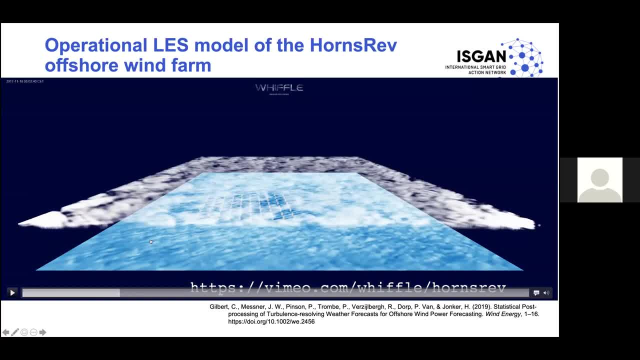 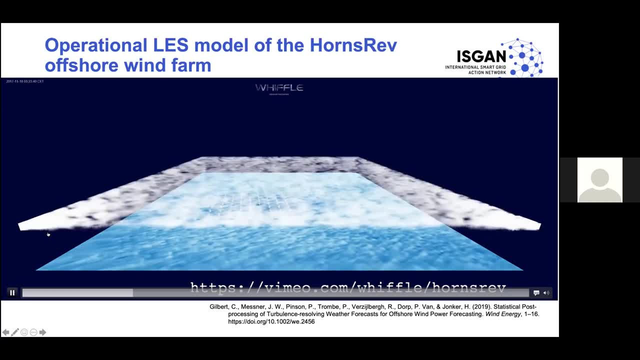 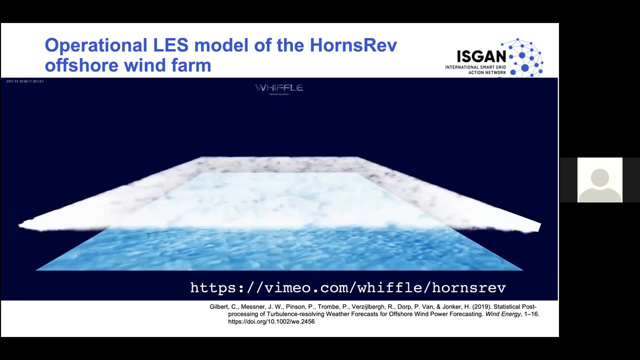 those are the wind turbine wakes. We also see some clouds moving through the domain. Let me just press play again. And what's the essence of a large eddy simulation model? Well, it's that it really explicitly models turbulence and cloud formation, like you see here. 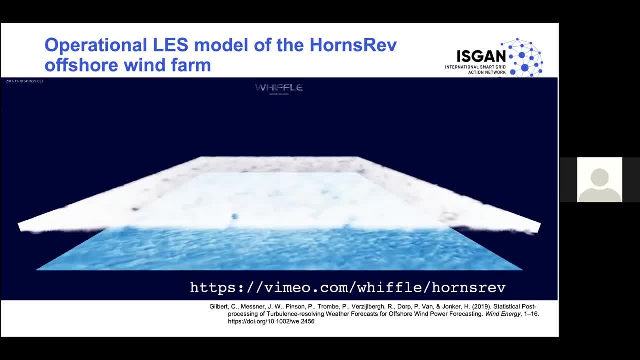 So all the different shades of blue that represents turbulence and wind gusts and that's all manifestation of atmospheric turbulence. And also in the cloud patterns you see small scale patterns. There's some sort of regularity there, but it's also some sort of chaos. 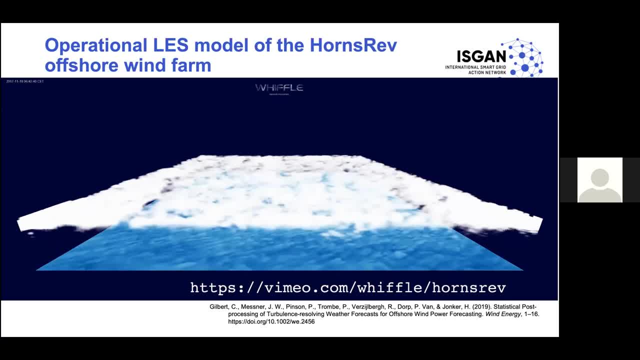 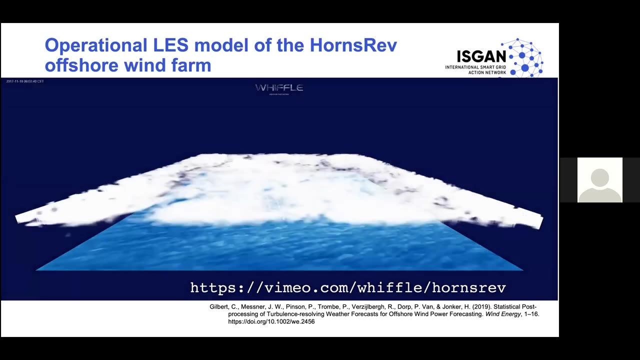 Well, these are essential characteristics of turbulence. So a large eddy simulation is really well designed to explicitly model the turbulence And this is really the strength of this technique. It's a computationally very heavy technique And we have partially solved this computational burden by doing the computations on a GPU, That's a graphics processing unit. 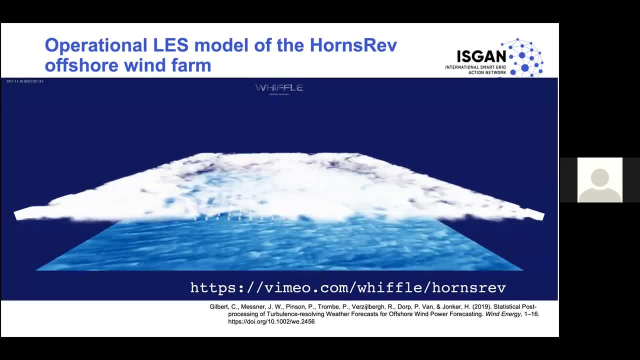 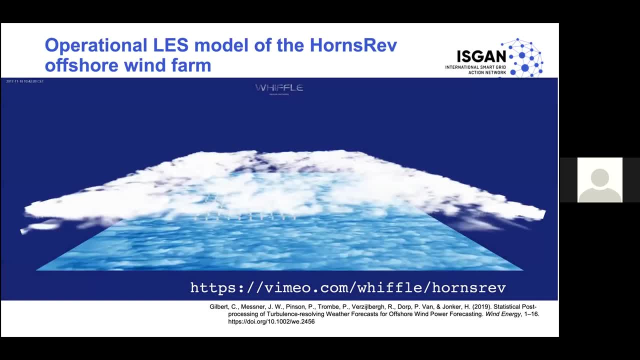 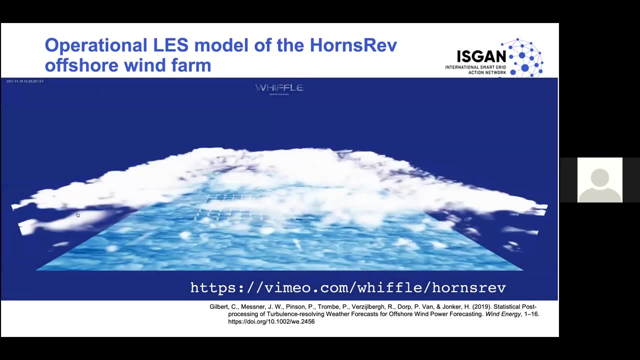 which can be very fast for parallel computation, And it has the additional benefit of well producing nice visuals, because after all, that's where the GPUs were made for, So you can relatively easily get beautiful animations like this one. So I go now into a bit more detail about large eddy. 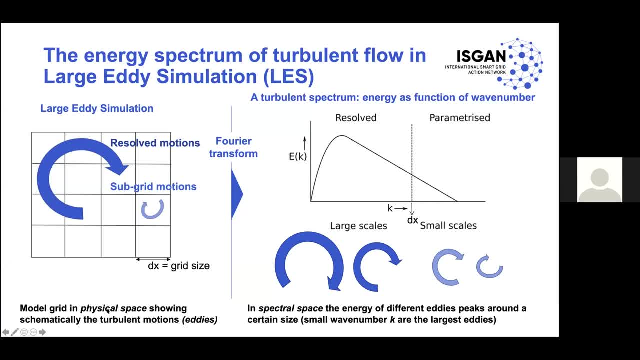 simulation. So on the left we see here, in a stylized way, the numerical grid of a large eddy simulation. and well, you see, the large arrow represent the resolved or explicitly modeled motions, and an eddy, by the way, is English for a turbulent structure, or whirl, if you wish. 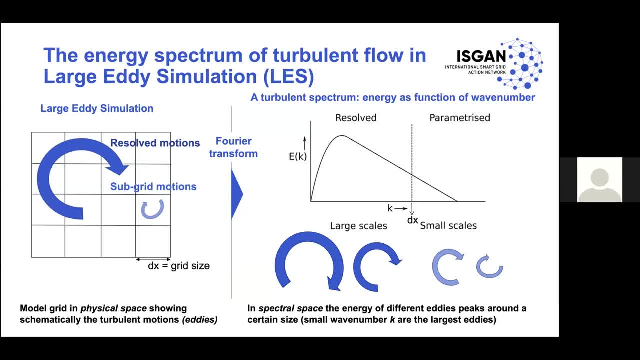 So the very essence of large eddy simulation is to capture directly the large eddies and then only parameterize the subgrid motions that are relatively homogeneous and their effects can be quite easily captured in a more stylized mathematical model. And if we now look to the 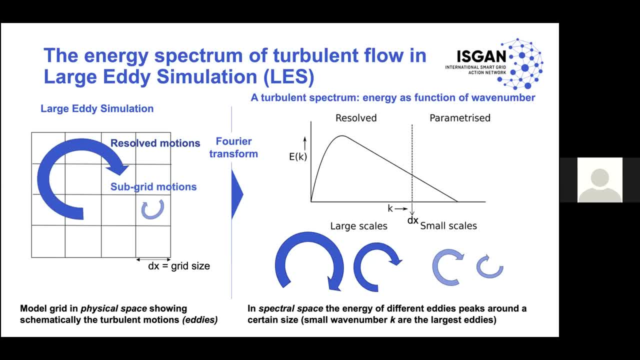 right, that's basically a different representation of the same. It's looking at the world in spectral space. So if you would make a Fourier transform of the physical space, then you can, for example, tell how much energy is contained in motions with a different length scale. 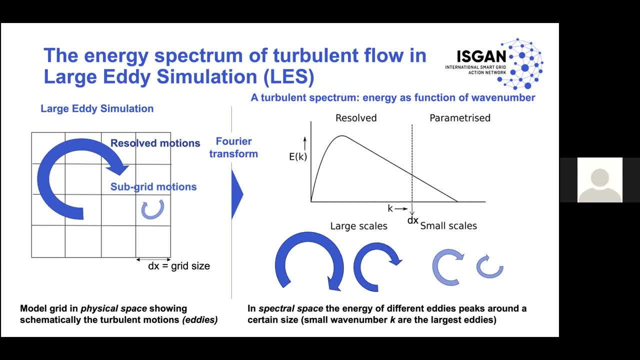 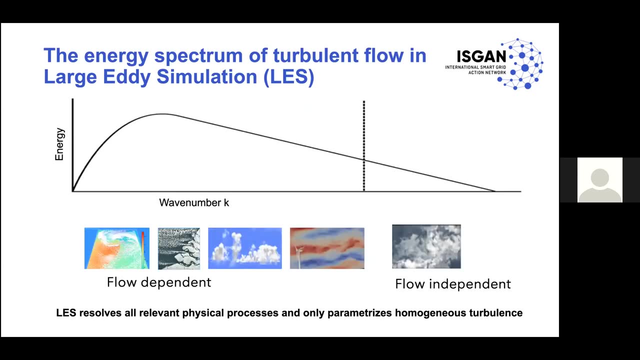 So on the left of this plot we see now the large scales and then on the right the very small scales, and only the small scales are parametrized, So the scales that are smaller than basically the grid size dx. So another way to put this is that large eddy simulation explicitly models all the flow dependent scales. 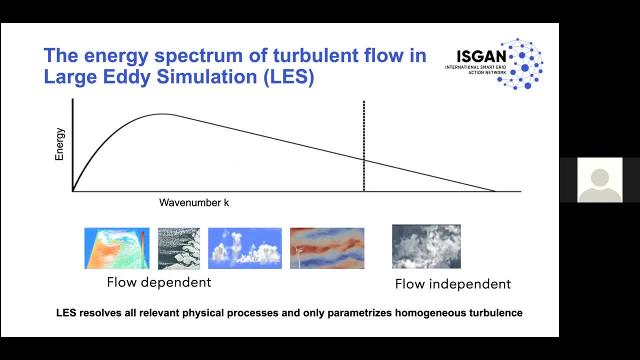 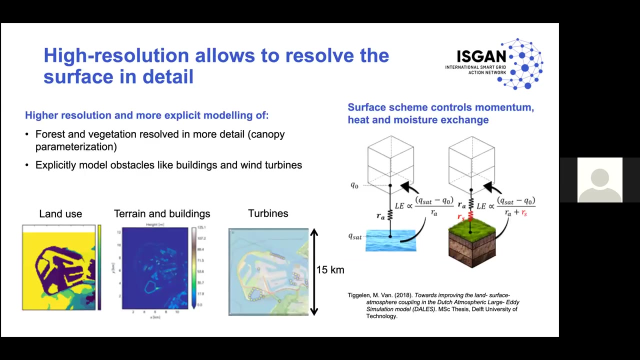 For example, scales associated with cloud systems or cloud streets, or even individual clouds, or even wind turbine models. So this is one of the ways to look at large eddy simulation, and large eddy simulation is then a method to produce very high resolution weather forecasts. But the high resolution except from 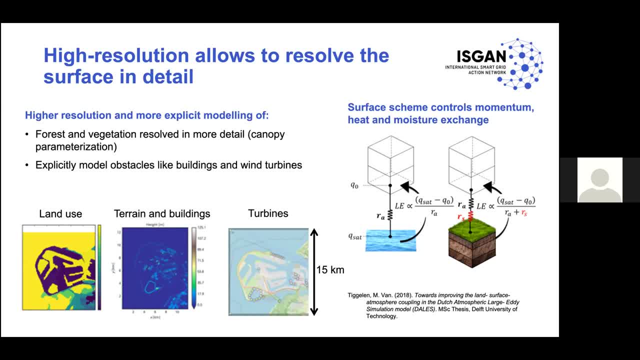 resolving all those turbulent scales and the clouds. it comes with some other advantages. It also allows researchers to take a closer look at the current data, So the very small scales from the left and the smaller scales from the right, and then also the smaller scales from the right, and then we can take a closer look at the 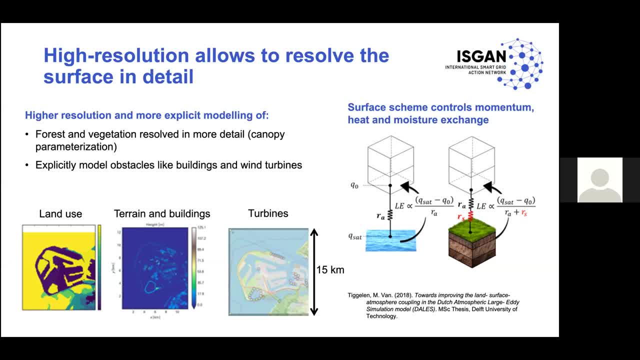 observation of the сделал data can be captured by the high resolution model and well, the interaction with the surface. that's well described in the so-called surface scheme. so the surface scheme basically controls how much momentum, heat and moisture is exchanged between well, the, the soil, the earth and the atmosphere. 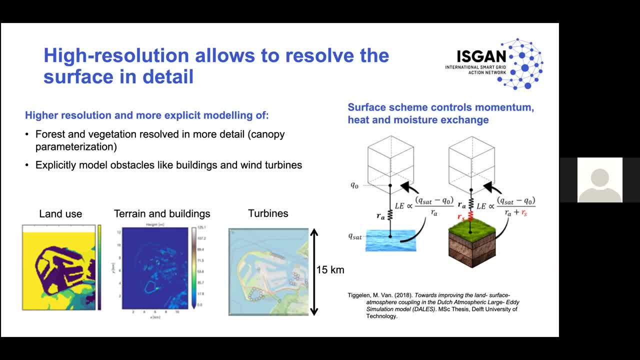 on top of it and typically these equations have some form. it's a bit like the well, the, the laws of in. in electrodynamics there's a difference in the quantity divided by some resistance that controls how much energy flows or how much humidity or temperature flows or momentum from. 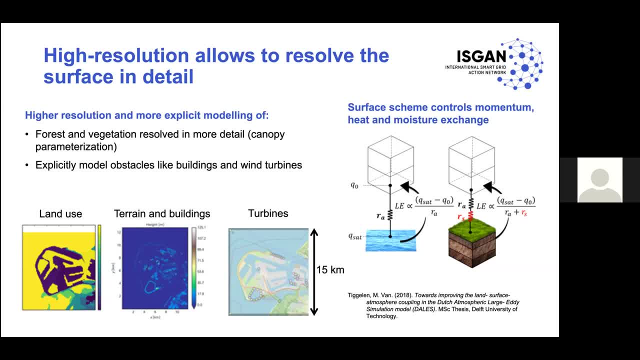 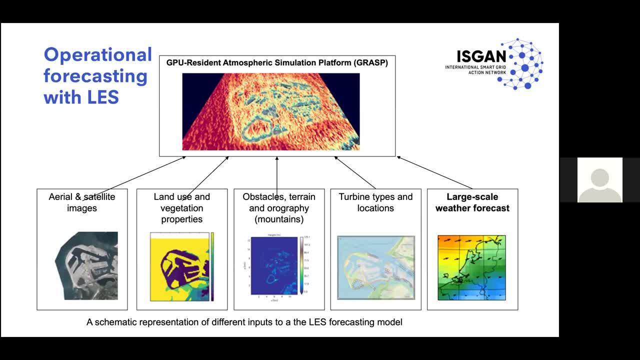 well, from the atmosphere to the earth or the other way around. so if we combine all this in a sort of schematic of how you do operational forecasting with large eddy simulation, so it requires a lot of input data. so on the left we have all the static inputs data, so the static 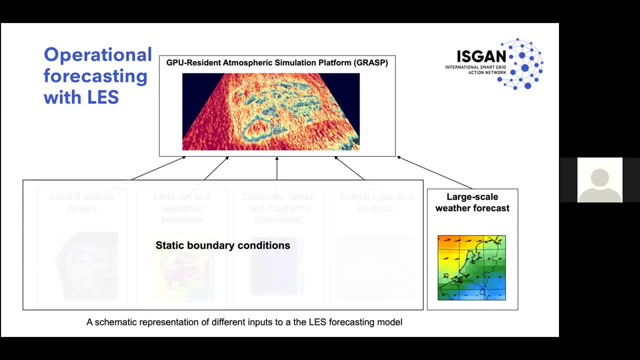 boundary conditions and also a dynamic boundary condition that comes from the large-scale weather forecast, because you saw in the animation of the horn drive wind farm that we only do a weather forecast for a very small part of the earth, so typically maybe 10 by 10 kilometers or 50 by 50. 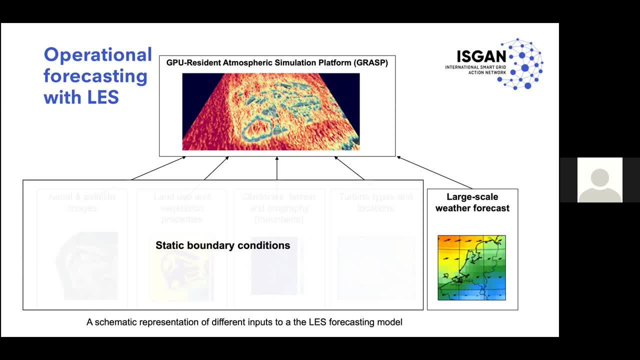 the weather around us is just a boundary condition for us. so we use the boundary condition from a large-scale weather forecast, for example the ones that are produced by meteo, france contents institute or other institutes. and well, we combine all this and use a lot of computer computing power. 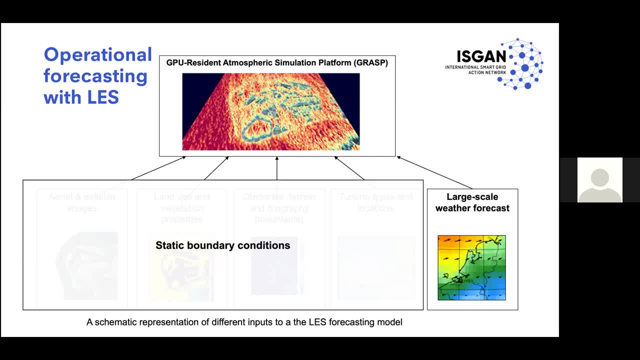 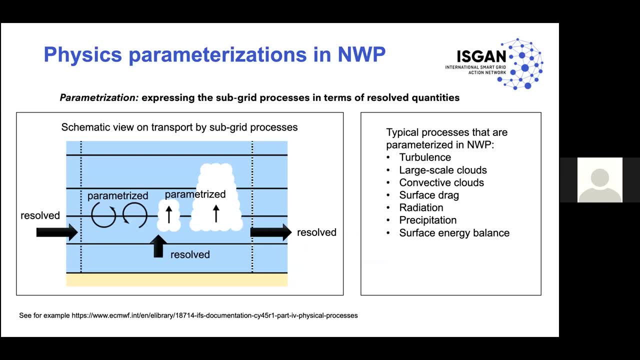 and then we produce the high resolution weather forecast. now to to shed a bit more light on on how this really differs from the traditional weather models, which are often called nwp- numerical weather prediction models. i want to say a bit more on parametrization content also. 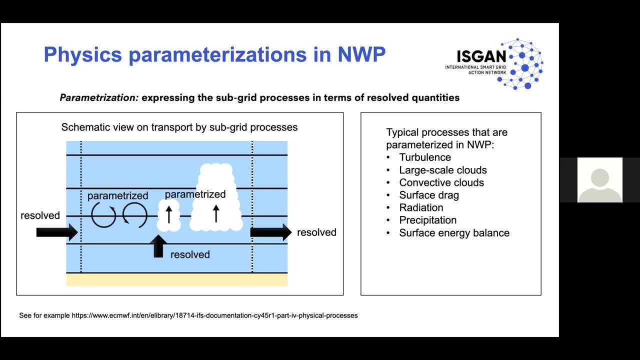 mentioned this. so parametrization is really, uh well, the art of expressing the subgrid processes that are too small to be directly captured in the numerical grid in terms of the resolved quantities. so that is, uh well, the the, the quantities that are resolved by the numerical grid. so, um, small. 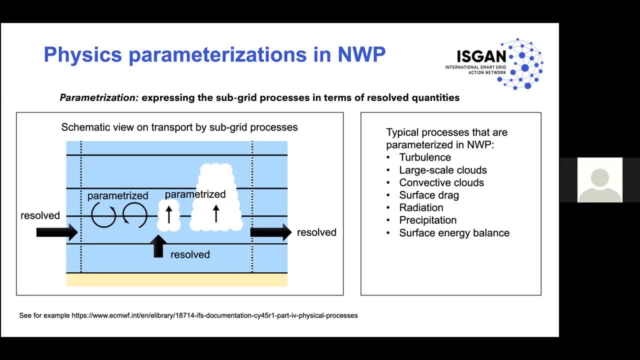 clouds are the ones that are being captured by the numerical grid, and then the other one is the. the metal grid is the one that has been captured by the numerical grid, and then on the left is the linear grid, and then the linear grid on the right is the linear grid. so that is also an example of 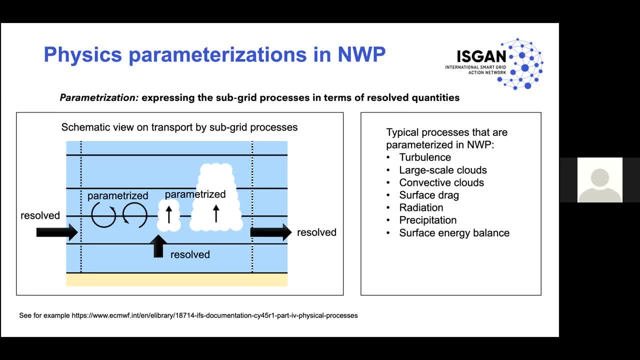 that turbulence. there's also an example of that. you see that here in the figure on the left, but there are actually many more processes that are parameterized. so here on the right we have a list. this is not even complete, but in these are probably the most important and they are very 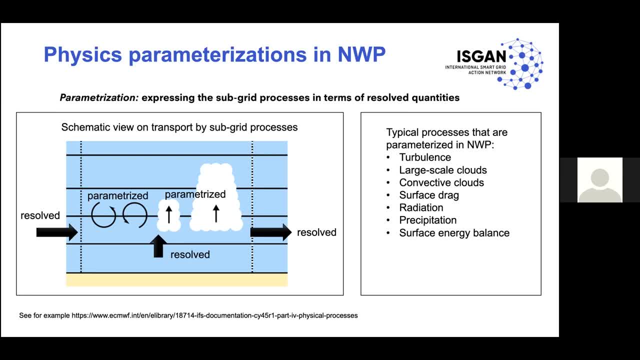 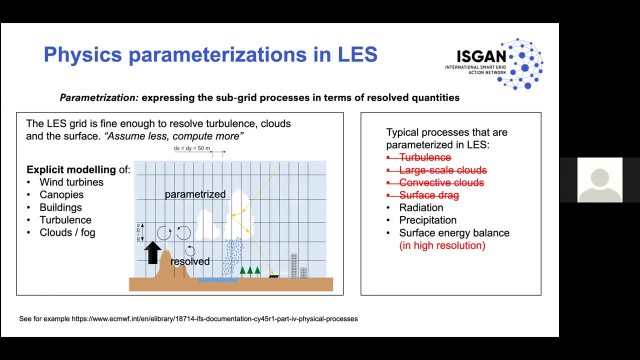 important for weather and they are also very important for well, the uh, the weather phenomena, the scale of economic activities. So a high resolution model, and then an LES being an example of that, that basically removes the needs to parameterize some of these processes because you can now directly represent them. 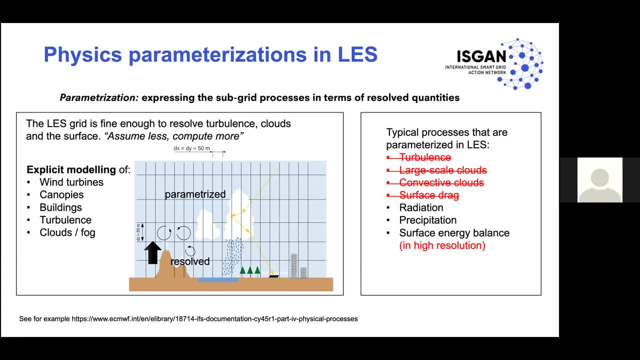 So here you could say: the philosophy of LES is really to assume less and to compute more. just throw in brute force computing. Well, you could say, to mimic the laws of physics that are valid in the atmosphere. So now you can actually explicitly model wind turbines. 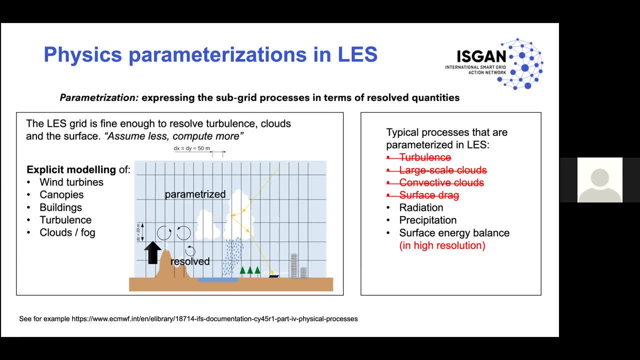 or canopies from trees or even buildings, and also turbulence and clouds, or a fog is a manifestation of a certain cloud and you can represent them in a much more direct way and therefore with higher accuracy. Now, of course, LES still has some resolution. 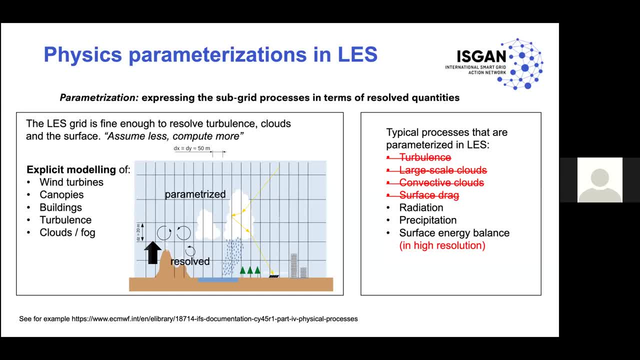 So typically we are talking about 50 meter. It can be a bit finer or a bit coarser depending on the application. So still, LES needs to make parameterizations. We cannot explicitly model individual raindrops or drops in the clouds, So therefore we still use the 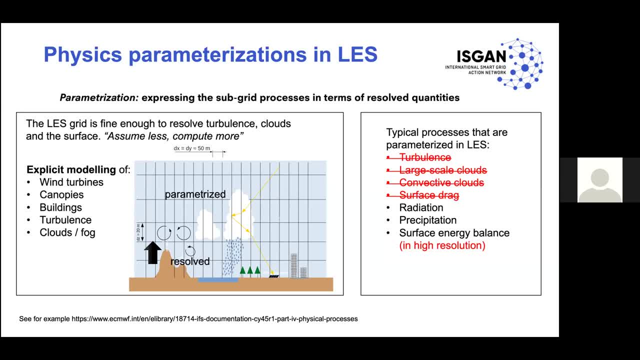 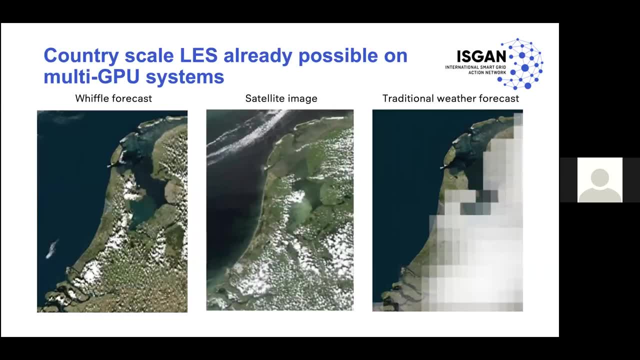 well, basically the same parameterizations that are used in standard weather models, but some of the process are now really captured directly. And well, to see what happens, what that does to a forecast, we can look at these pictures where we use a lot of GPUs in parallel. 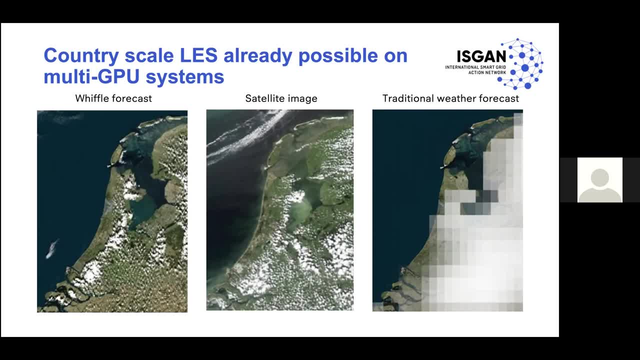 to do a large eddy simulation over an entire country. You see it here on the left Now, in the middle is the satellite image of that day And on the right is the traditional weather forecast, And you can see that. well, large eddy simulation gives a much more realistic look. 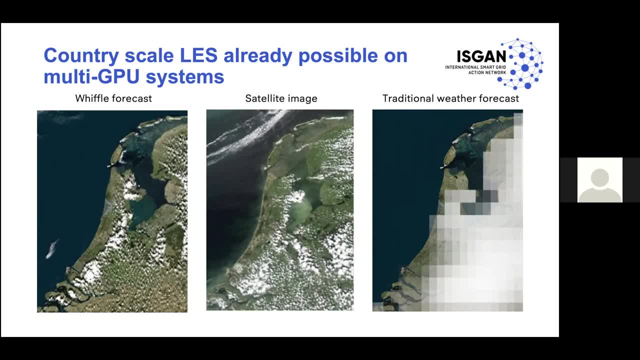 and feel of the clouds. It captures certain details Like the cloud size distributions or the vertical structure of clouds. That's really difficult for the traditional weather models, Although they are really pretty good on average, they just do not have the resolution to capture some of those details. 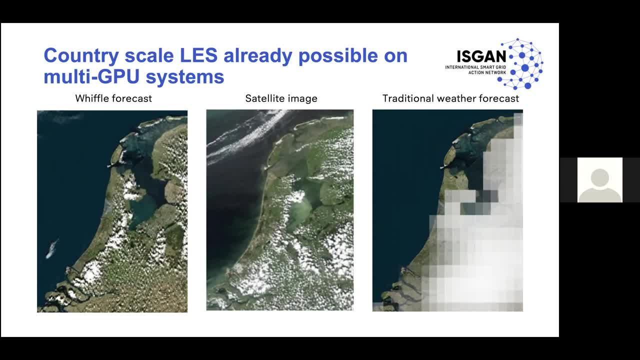 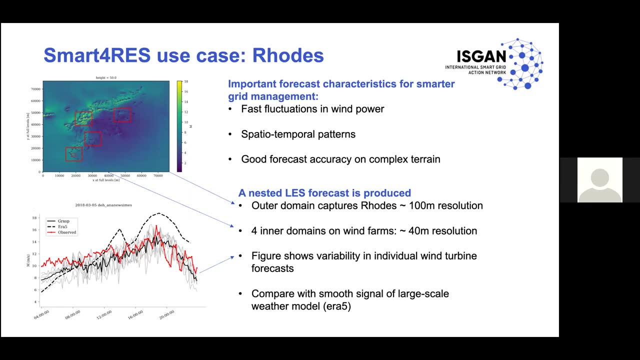 which, as we saw also from Mattia's presentation, can make a lot of a difference for renewable energy applications. So in the Smart4US projects one of the use cases where we use large eddy, large eddy simulation for is for grid management. 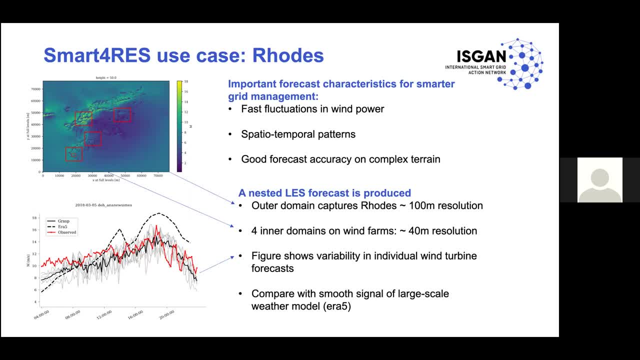 on the island of Rhodes. So well, you see here on the top left actually, a wind speed map of the island of Rhodes. It's- yeah, it's roughly 60 by 60 kilometers large And you can immediately see that the mountains on the island. 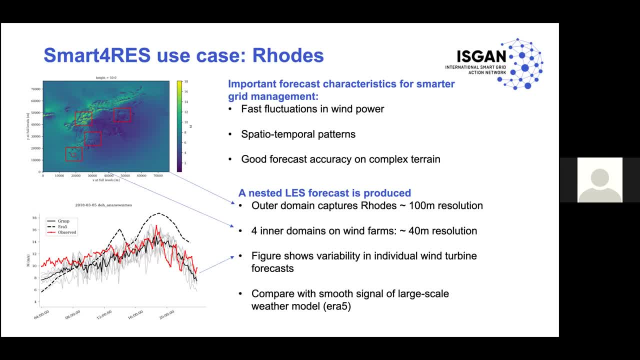 have a significant effect on the wind. You can clearly see the signature of the wind there, And a high resolution model allows you to capture some of those details. But apart from the, let's say, the spatial details, there's also the temporal fluctuations. 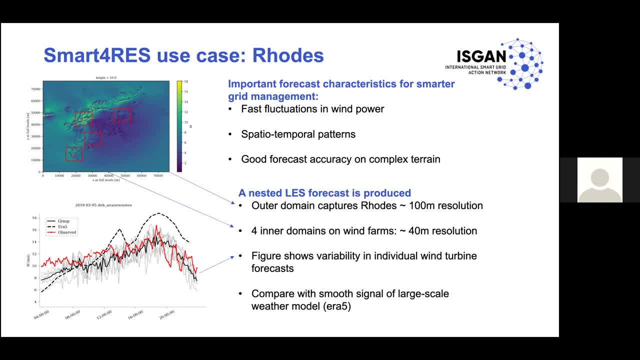 Quentin also showed a few examples of that, But large eddy simulation can well can produce even more detailed results And also the well the spatial temporal correlations. they can actually be important for this application of grid management. So what we have done and what we are still in the process: 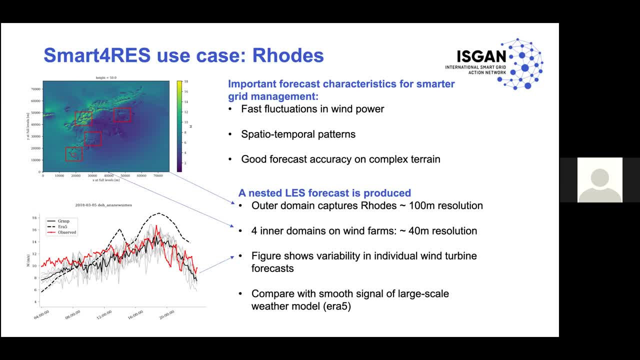 of doing is to make very detailed simulations for four wind farms on Rhodes. So the four rectangles in the figure they show the location of the wind farms And then we're zooming in on one of them in the bottom left figure. So we have set up basically a nested simulation. 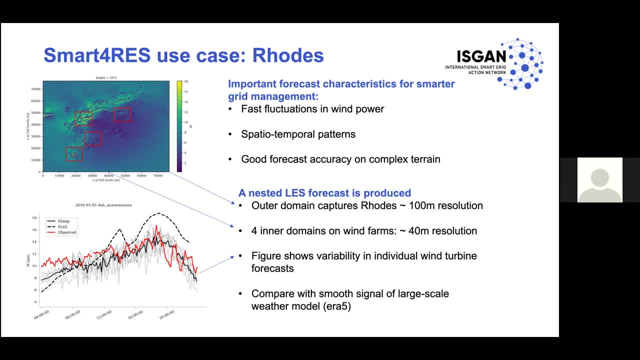 So we do one forecast for the entire island of Rhodes, a typical resolution of 100 meters, And then, within that forecast, we do four inner domains. You could say it's like a zoom in or a magnifying glass, That's on even finer resolution, on 40 meter resolutions. 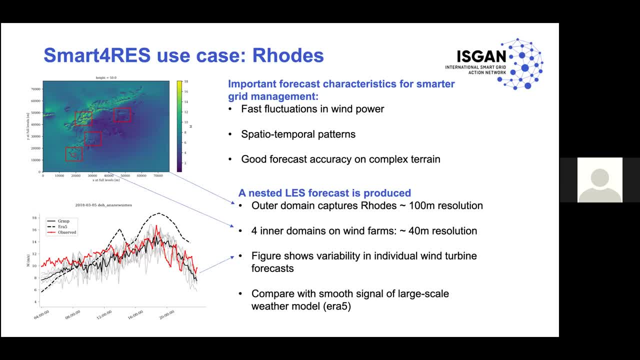 And then really you capture some of the complex flow phenomena that are, for example, occurring around a mountain ridge. This is usually where the wind turbines are located. And also, you see, in the bottom left figure, that's the light gradient, That's the velocity lines. 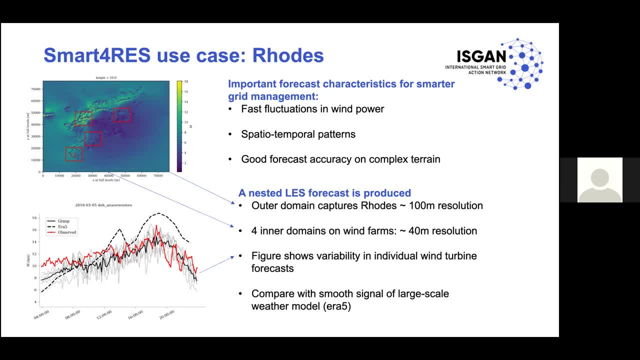 They denote wind speed at individual turbines forecasted by the model And you can see also the fast fluctuations. And if you compare that and the black line is the average for this particular wind farm, and if you compare that to the red line, which 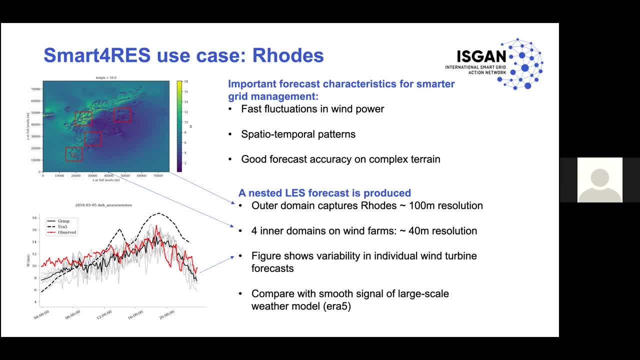 is the observed wind speed at this wind farm. you see that well, it captures it pretty well. of course The fluctuations do not map one to one, But the typical size and the velocity line, which is very low. So the left line is the average for this particular wind farm. 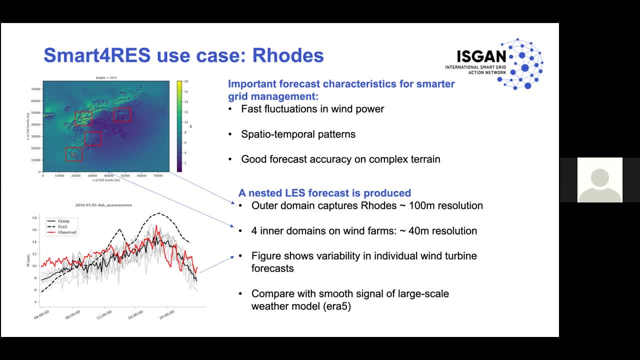 And the right line is the red line, which is the observed wind speed at this wind farm and duration of fluctuations is well captured by this model And if you compare that to the dashed line, which is a large scale weather model, then you can see that it has a much smoother output. 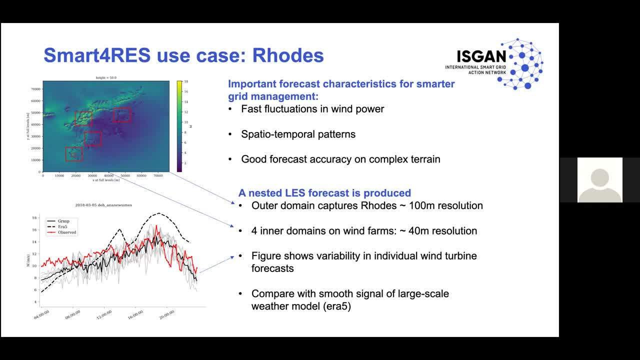 So this will not give you much information about the typical fluctuations. So, apart from using this high resolution forecast and doing all kinds of advanced decision-making with it, that's basically up to the other partners in the Smart4Rest project. We are also working on some innovations. 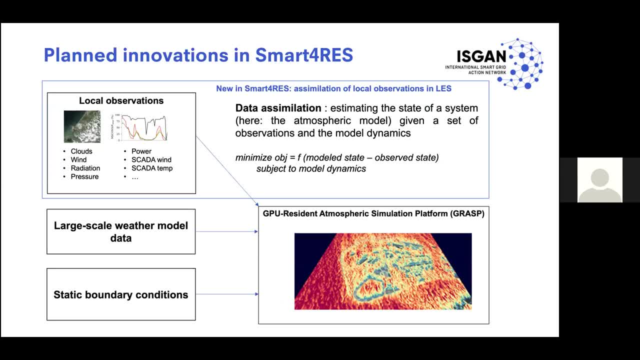 in the high resolution modeling itself, And this is mostly related to what we call data assimilation. And well, you could loosely describe that as a fusion of observations and models or, a little bit more formally, as estimating the state of the system. So in our case, the atmospheric model. 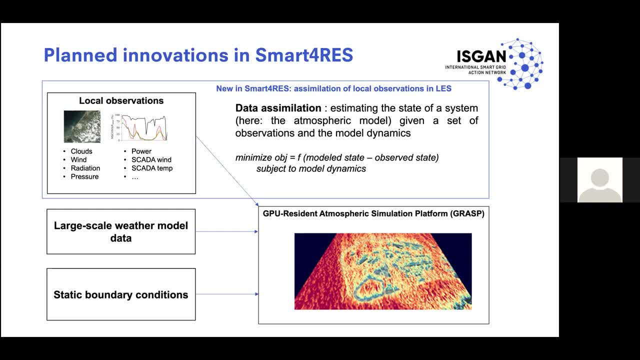 given a state of the system, a set of observations, and also given the model dynamics So well in mathematical terms, we are trying to minimize some objective function which is a function of the difference between the model state and the observed state. 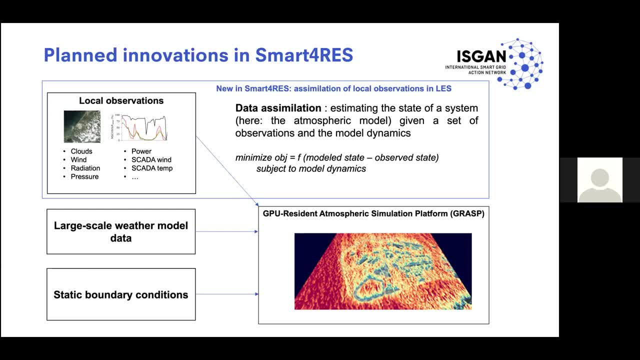 but subject to the model dynamics. So it really combines. it tries to combine the best of the models and local observations. So you can think about meteorological observations like clouds, wind, radiation, pressure, and then well, these come in more traditional forms. 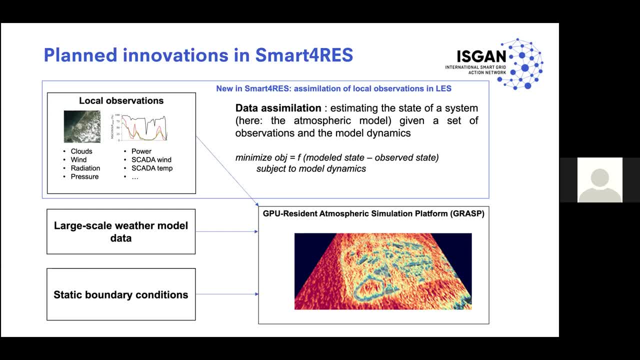 for example satellite and ground stations, but also more advanced forms like sky cameras and LIDAR measurements. But we can also use the measurements of the wind farms or solar farms themselves, because our model is fine enough to actually represent those wind farms in the model. 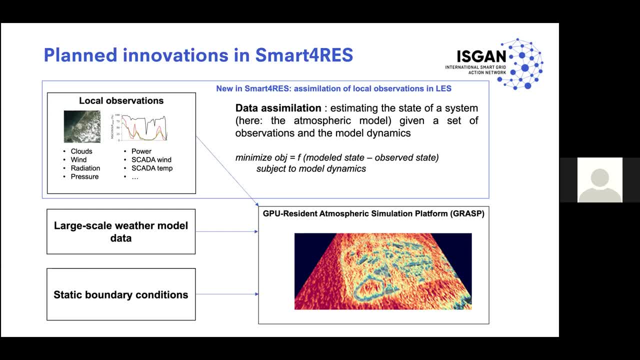 We can also use those observations to basically estimate. we estimate the initial state of the atmosphere and then use that as a starting state to well to produce the forecast from. So summarizing compared to what we have already is using static boundary conditions. 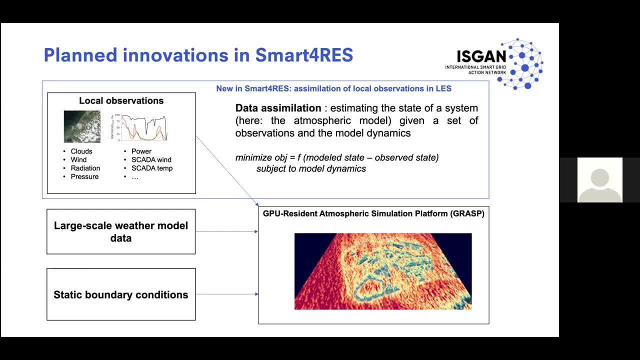 and large scale weather model data. We now also want to use local observations and combine those three to make better short-term forecasts. And you can imagine that using local observations will especially benefit the short-term forecast because obviously, well, our weather for a few days in advance is not. 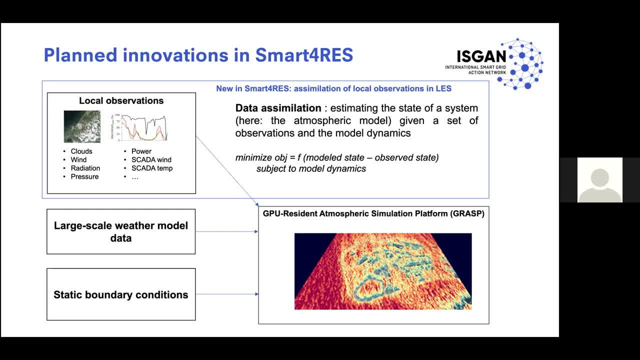 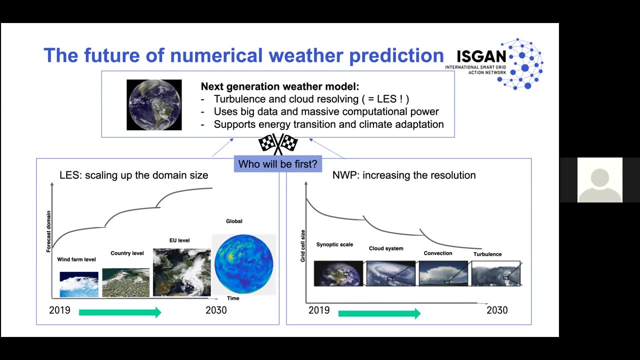 well made locally. it's further upstream, if you wish So. for this we really expect benefits for short-term forecasts. So let me move now a bit to the further future. These are not all things that will be addressed in the Smart4S project. 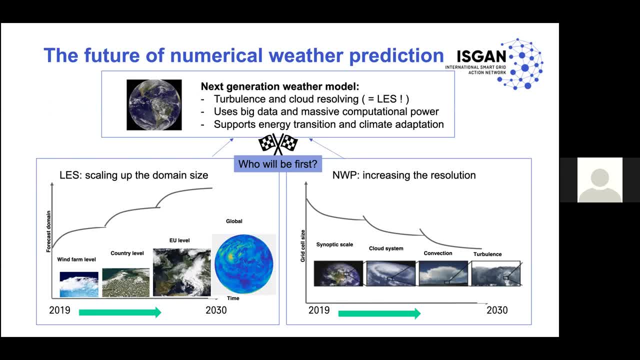 but well, I think we can conclude from what Quentin has been telling you and from what I have been telling you that there are now two approaches to weather forecasting. So there's the very high resolution, large eddy simulation approach, And for us it's a challenge to scale up these forecasts. 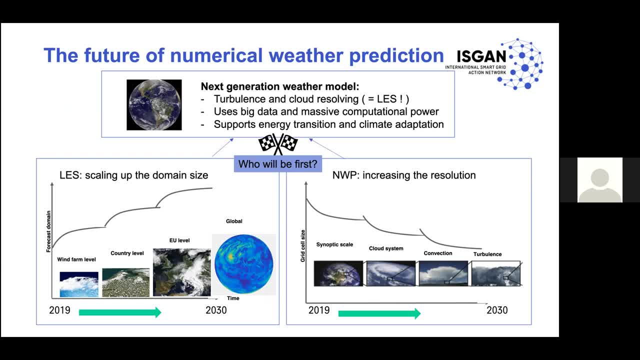 So we are using more and more computing power to increase our simulation domain. So we go from wind farm levels to country levels and maybe even to European level or global level at some point. And the traditional numerical weather prediction models on the right. 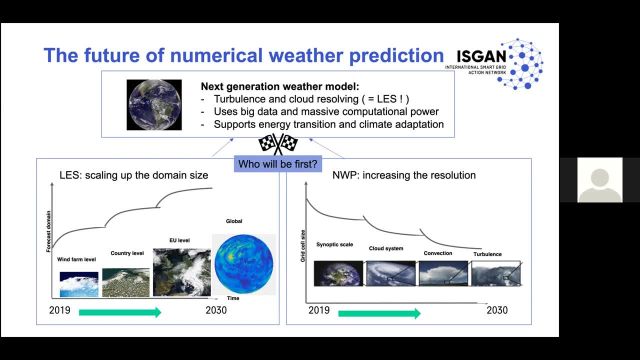 well, they already cover the entire globe, or at least the continent, and they are refining their resolution ever more and more, So they start picking up processes that, like cloud systems and convection that's, currently are still parametrized but then will be directly resolved. 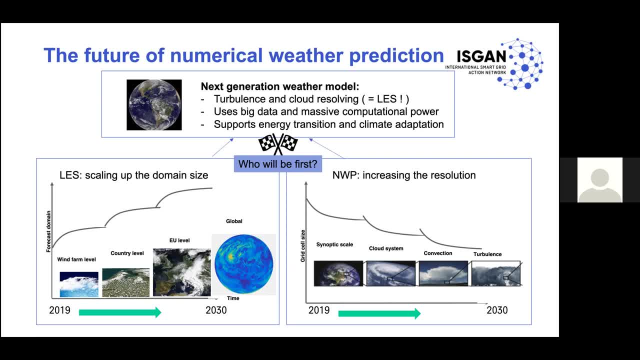 So you could see this as a bit of a competition: Who will be first The bottom up approach- LA-S- or the top-down approach- numerical weather prediction models? And well, it doesn't matter who wins, but the next-generation weather model will be a turbulence and cloud-resolving model. 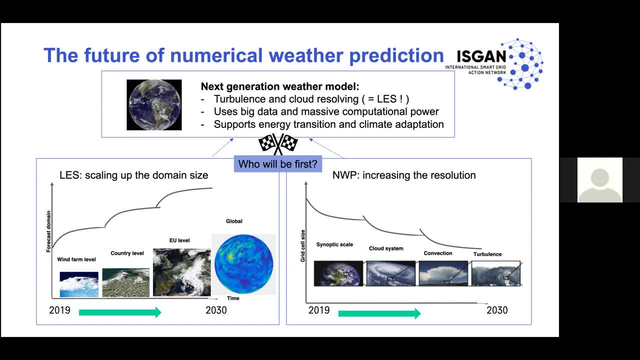 So in essence that is a large eddy simulation. It will use a lot of data from observations and massive computational power, and it will have an important role to play in the energy transition, but possibly also for climate adaptation. So it brings me to one of the final slides. 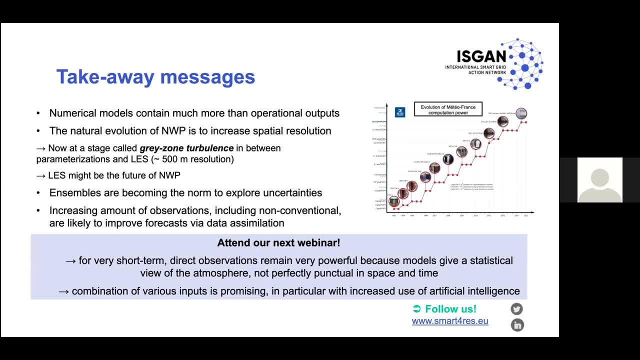 This is a bit concluding. So well, we've shown today how numerical models really well contain a lot of physics, much more than what's normally operationally outputted. And well, they become ever finer And we are reaching a zone where which is sometimes called the gray zone. 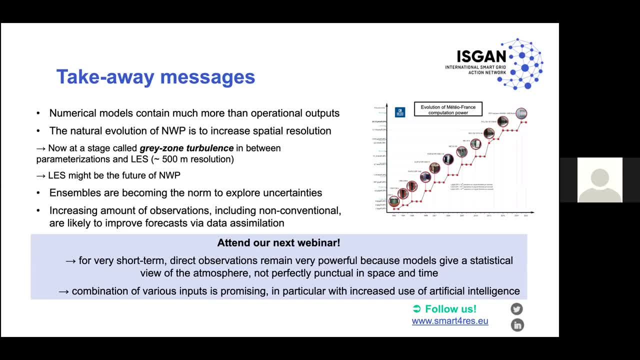 or the terra incognita, or well, unexplored territory, Where well, basically, a sort of convergence between the traditional weather models and the turbulence-resolving models, And well, this is a difficult zone and here are scientific challenges for us. 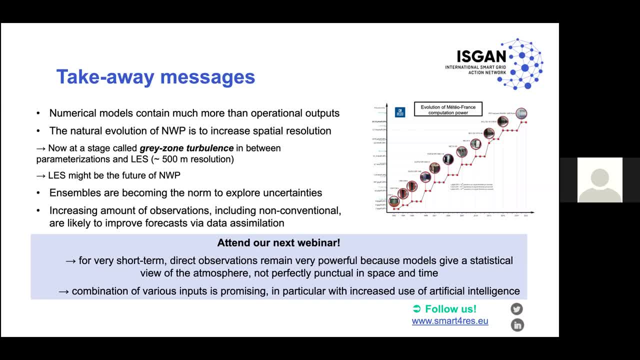 Well, content also shows the power of ensembles to explore these uncertainties. And, yeah, we see on the right here how the increase in computing power helps us. So this is both on the traditional, So this is both on the traditional computers as well as the well modern GPUs. 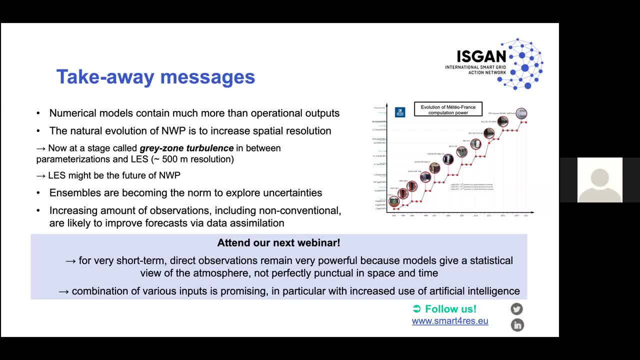 so the graphics processing units. That helps us to address these challenges and go ever finer. Yeah, and we are also helped by, well, the increasing amount of observations. So that's conventional but also new forms of observations, And they will help us improve the forecast further. 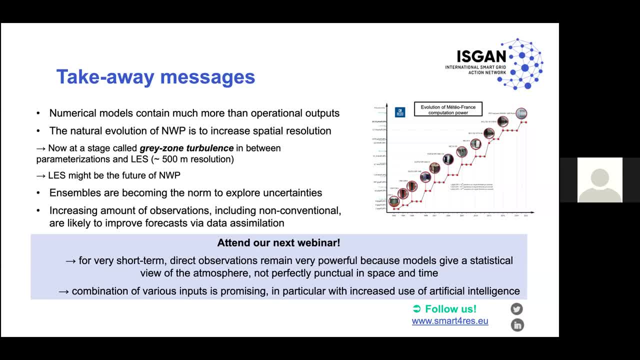 Now the observations are also the topic of the next webinar. So there our colleagues will talk about well advanced ways of observing the atmosphere And also what we will do with that in- yeah, in- our weather prediction models. So there are some further reading. 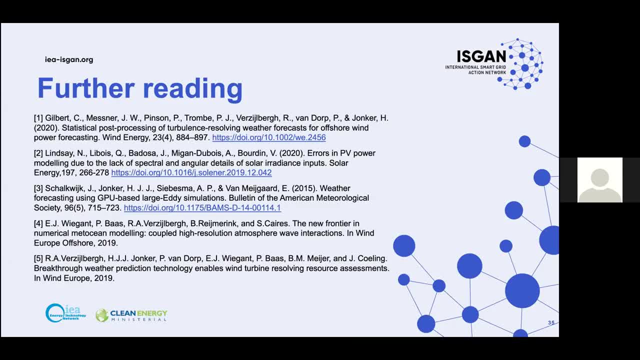 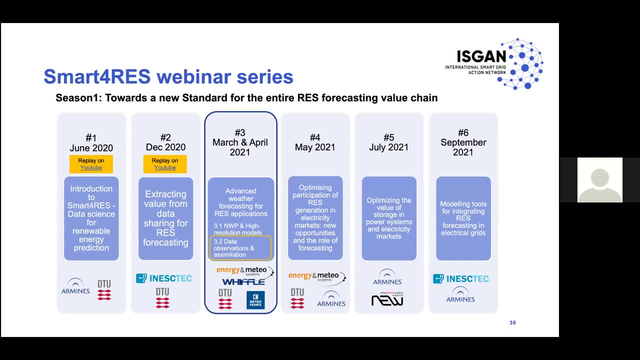 You can look at this in your own. time Brings me to the last slide. So we had today webinar 3.1.. The next one will be somewhere in April. It will be about Data observations and data assimilation. It will be presented by our colleagues from DLR. 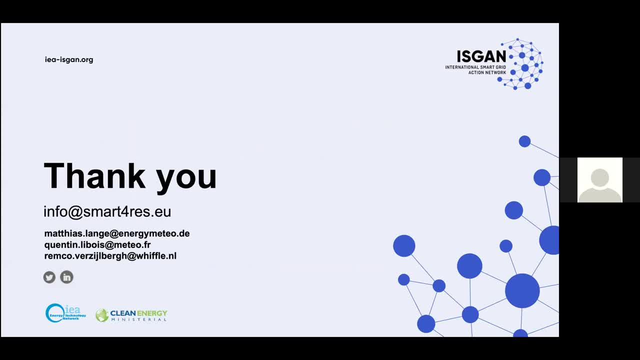 And I think this brings me to the final slide. So I want to thank you for your attention And I'm not sure if there are questions. I am sure there are questions. Actually, I see it on my screen, So I think we will go through them.